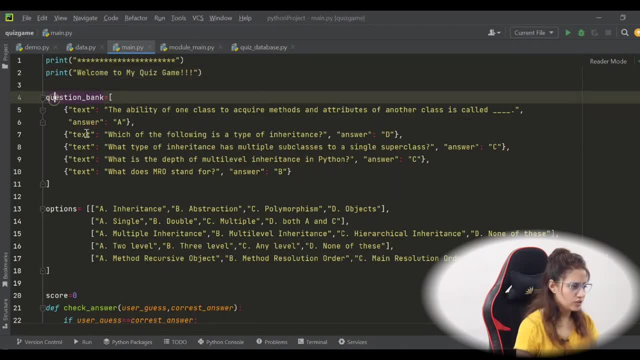 see, this was a project for our quiz game. we have question bank and then we have the answer of these question here And then we have options A, B, C, D for each question. we have only five questions, we have taken only five questions And the code is also in this. 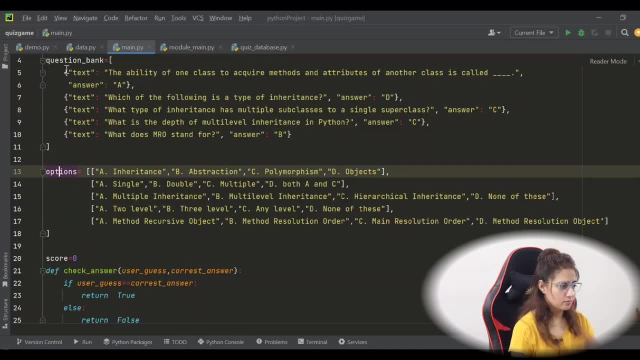 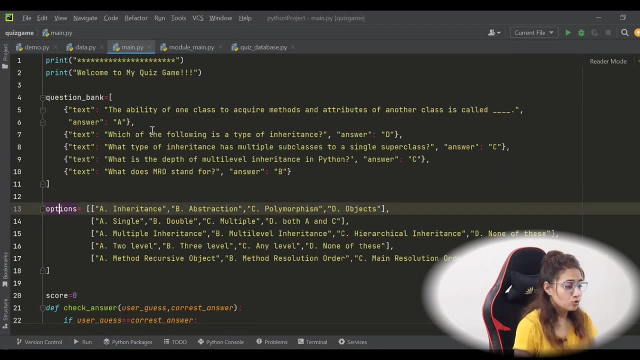 file, only in one file we have everything, our database. obviously this is what kind of it's a database for us, right? So data as well as the main coding, right? So if I want to add more questions, if I just want the, in my quiz there should be 50 questions, So the question. 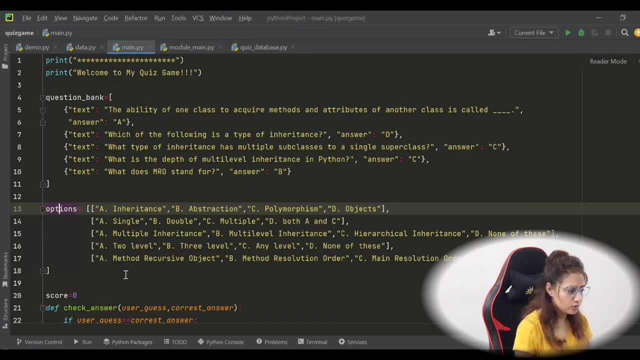 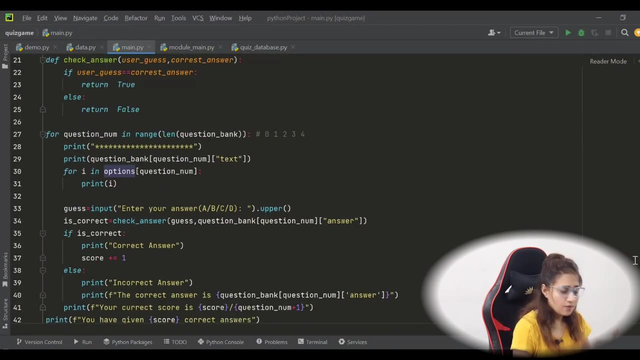 question bank. it should be 50 questions there, then optional, So there should be 50 list of having A, B, C, D options for everything, right? So the program or this program would be very much readable because in the same I have database and then here after that I am having the main. 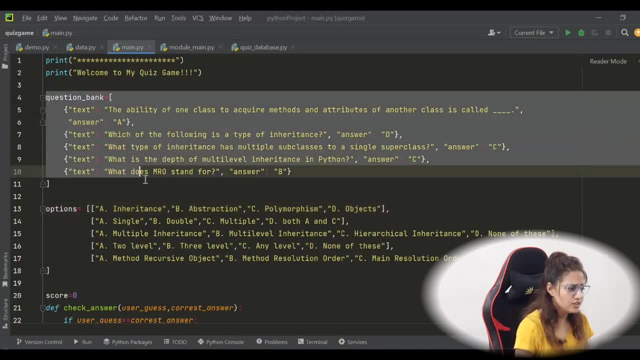 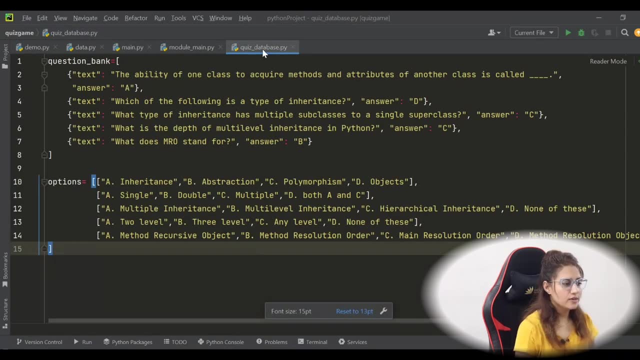 code. So the better option is what? what we can do? we just take this database from here. we just create a new file that is quiz underscore database, dot py, And this is our file. this file is having this data right. So this database. Now, if you want to use this database in our main, 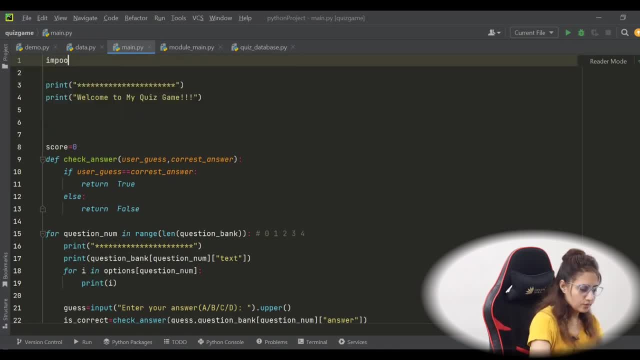 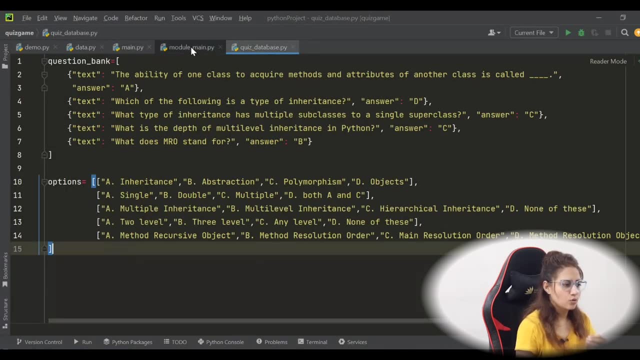 file, then what you need to do? we just have to import. how do you have to import different modules? So just use import keyword and the name of that module. That's it. quiz underscore database- right, quiz underscore database. That's. 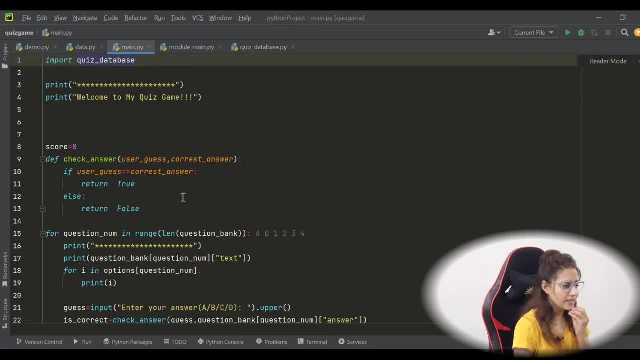 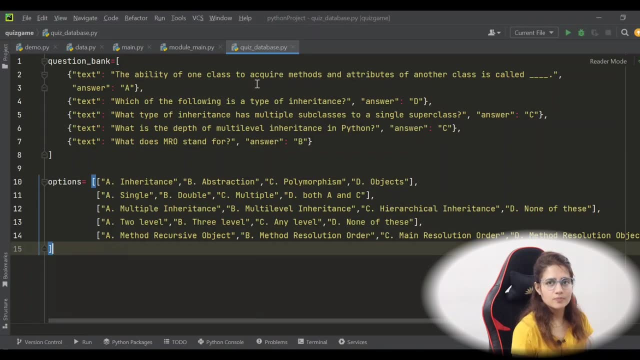 it. Now this database we can use in this program. So I think that is more readable now, more manageable, right, So now this separate. this file is what? it? just a module. So in Python every file acts as a module. So what we can say? 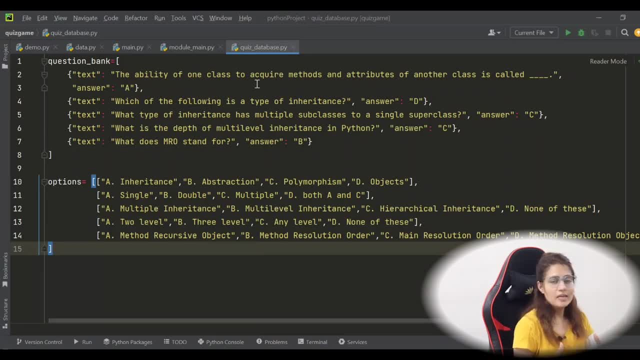 what is a module? the definition of module: it's just a file having or containing some Python code. you can say, like some statements, variables or definition of functions or classes, anything it can have right. So that is simply a module. That's it Right Now. if two, two, 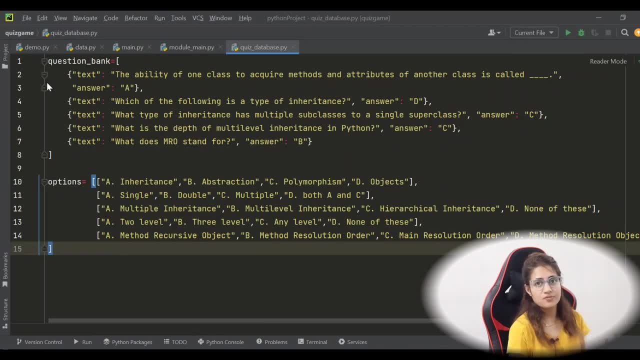 you know, people are working on the same project so just like me and my friend, so I can give this file to my friend- question bank file, this database file. I can just say I want 50 question or 100 question in this database. So he or she is going to update. 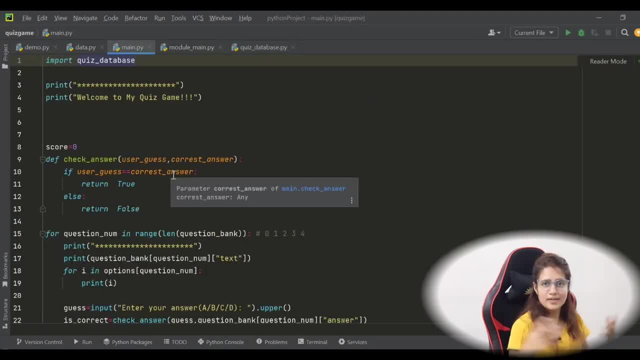 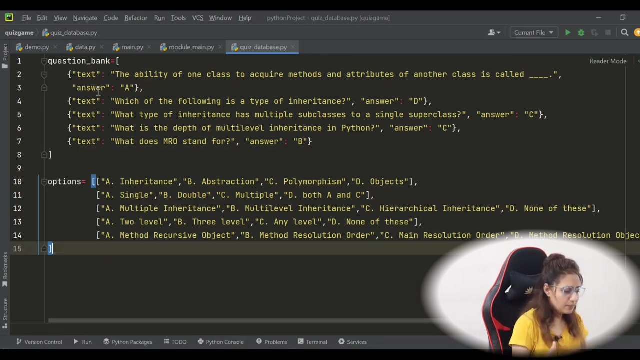 this file only And right, And in main file. there is no need to update anything. I just have my main file and after updating this, main file will work as it is. So there should be no change in the main file, Right? So this is how, if you have divided your project into different files- multiple- 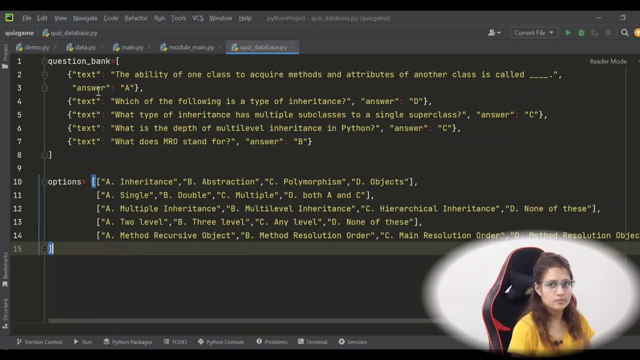 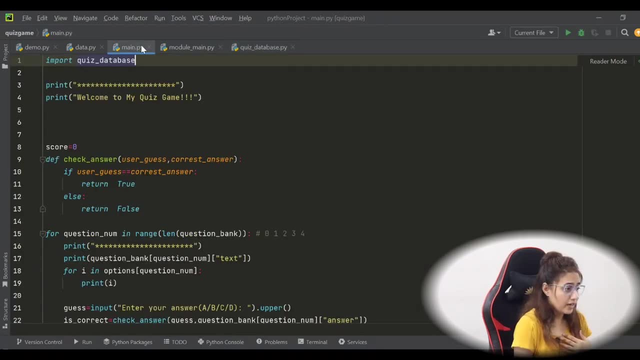 you know, more than one people can work on that project, Like then right now, in one file in data base. my friend is working in main file. I'm working right If I have only one file- mainpy- and everything is within that file. So only one person at a time can work on that file. 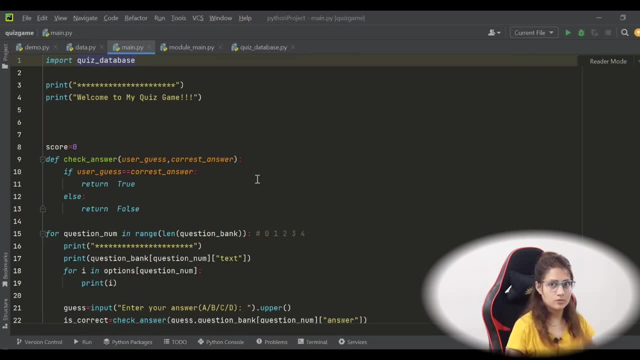 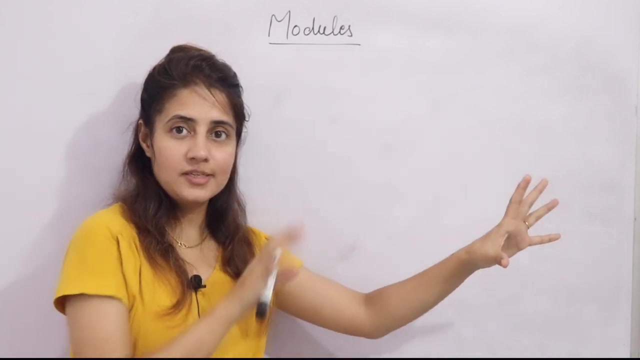 right, Not two separate person or more than one person. Okay, So this is what concept of modules? So now, first let's discuss why we need modules. this concept So, as you have seen, after dividing our project into two separate files, like one is for database and one is a main file, 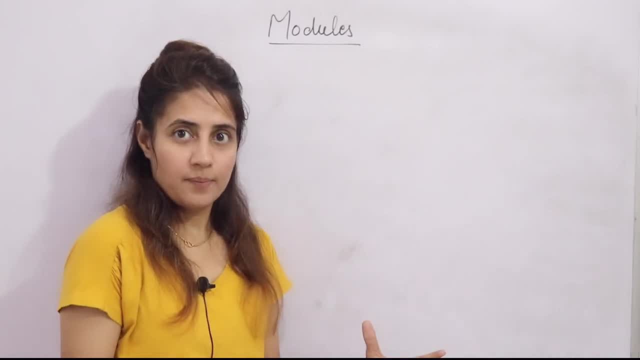 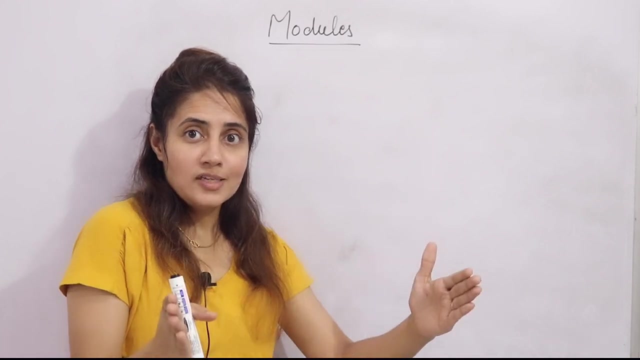 Right, That was easy to manage our program or our project, Although we have divided our project into two files only because that was not so much big project, or we are having a small program. only that was not so much large, Right. But yeah, after dividing into two files, that was, I think, more. 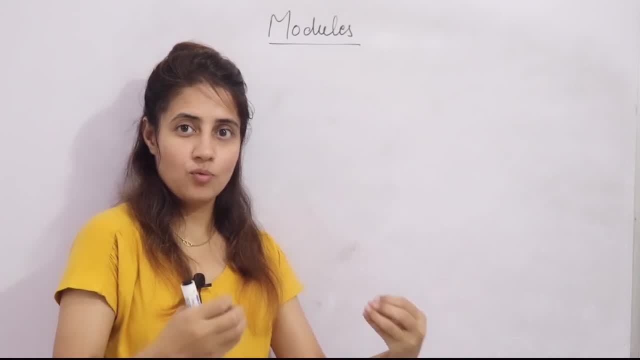 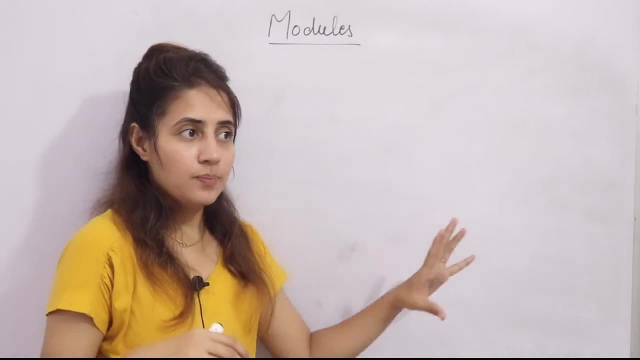 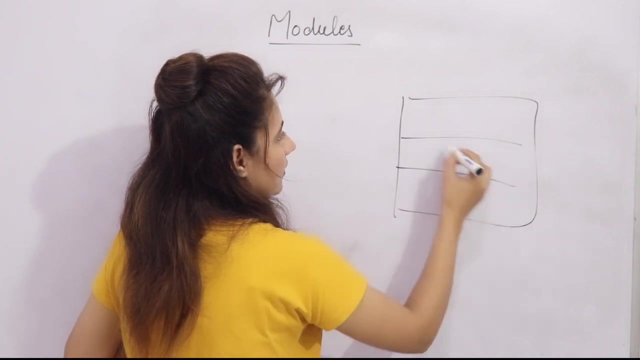 manageable right More readable. So that is what. what first reason to use modularity concept or to use modules in Python? Or we can take a real life example. Suppose see, we have a almirah or we have a wardrobe And I'm having like maybe multiple. 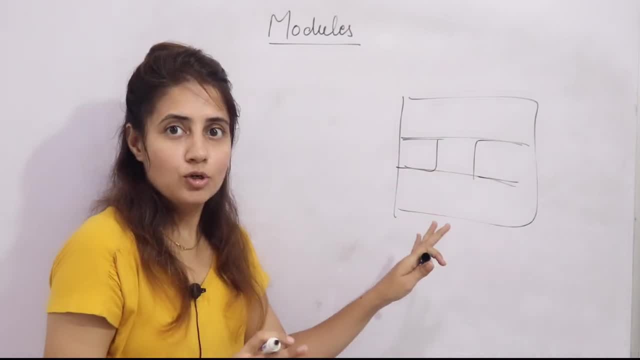 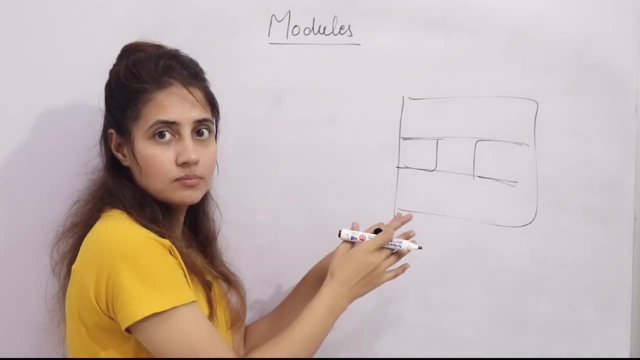 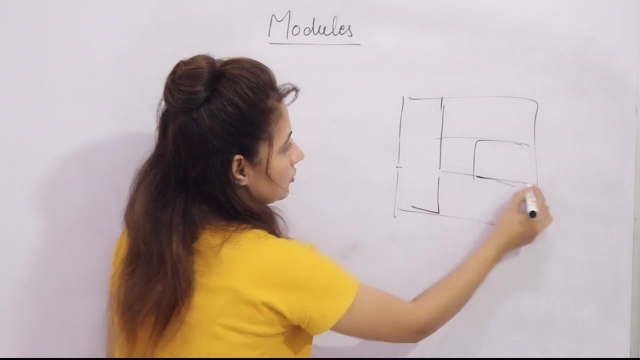 you can say shelf in my cupboard. So I have like t shirt, tops, jeans and everything. So I'm putting everything, I just fold my t shirt Right And here is suppose I have this one, this shelf, So I'm just putting my t shirt here, then I'm putting my t shirt here, then I'm putting my t shirt here, then 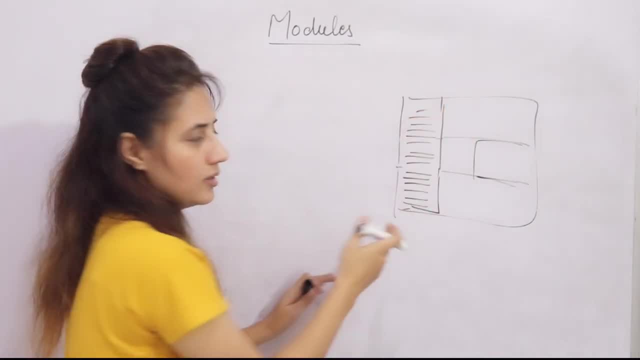 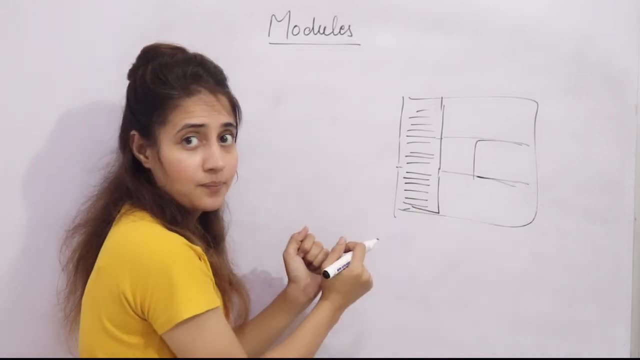 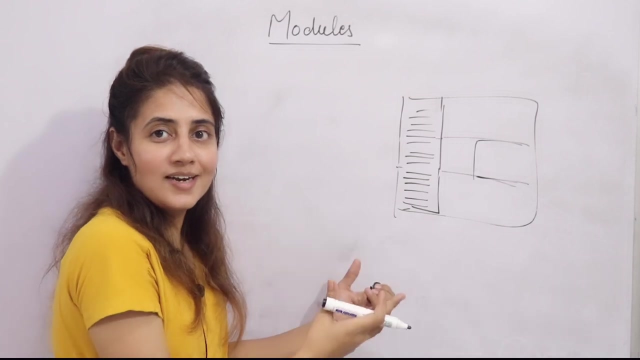 I'm putting my jeans, my pajamas, my tops and everything in just one pile, Right? So if I want to pick that one top which is here near the bottom, then if I pull this out from here then everything will be messy again, Right? So better idea is what just separate out, like my here I'll. 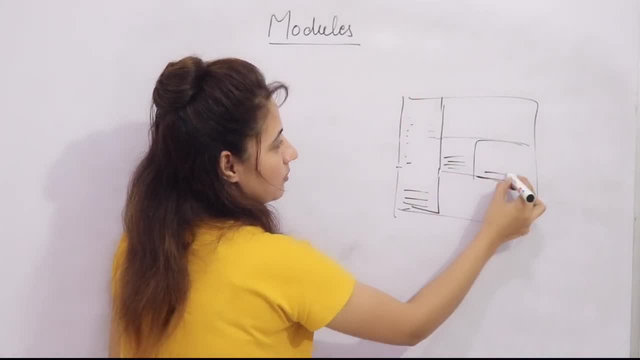 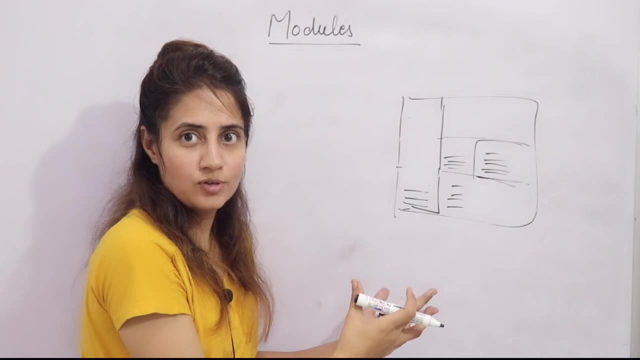 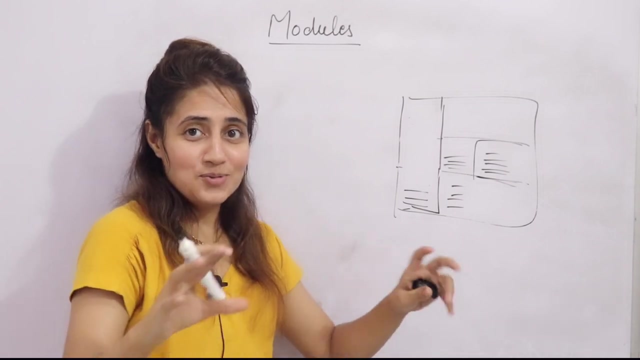 put my only tops and this I'll put my jeans, my pajamas and like this. So now it would be easy to manage my clothes, it would be easy to put the clothes, to take the clothes from the almirah and all right, I hope you are going to. you're able to relate this example, right? Same same thing. 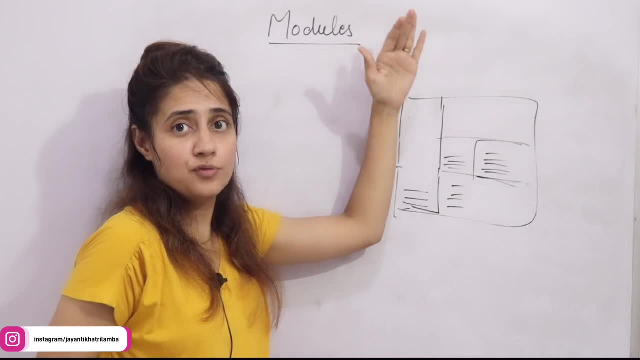 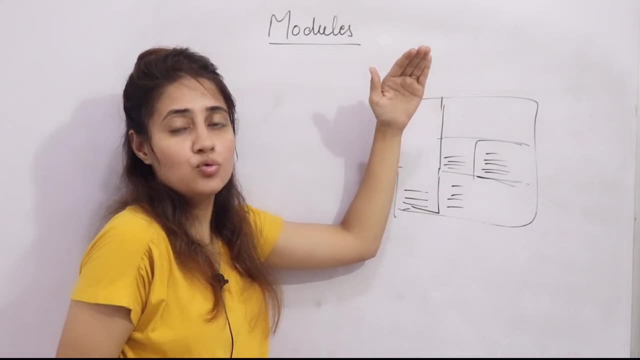 if your program, like, gets bigger, many lines of code, then rather than putting all the lines or everything in a single file, because that would be not easy to manage that program, right? We just split the program into separate files, Right? So that would be easy to manage. my clothes it would be. 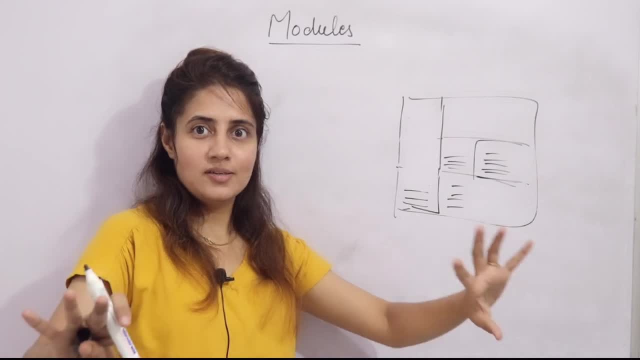 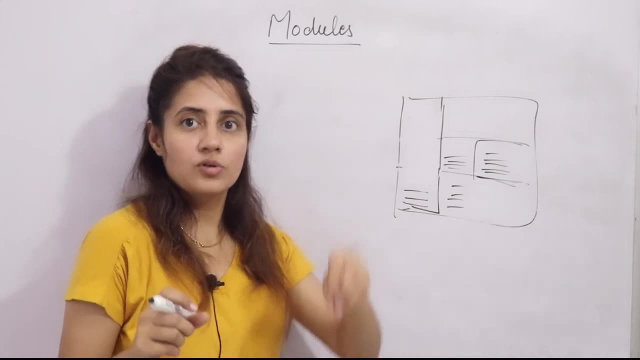 easy to manage my clothes. it would be easy to put the clothes, to take the clothes from the almirah and all right. and that would be very easy after that to manage those files, because whenever you want to use any file then I can import that file. right, How we are going to import that also, I'll 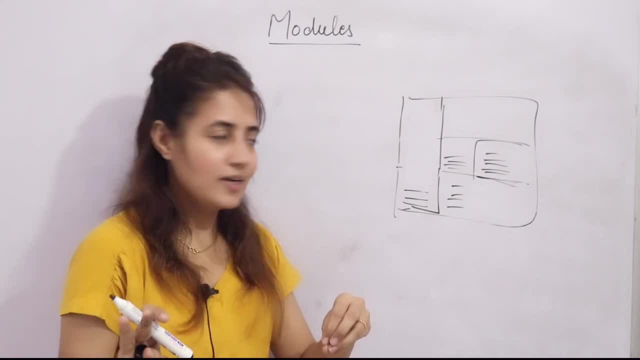 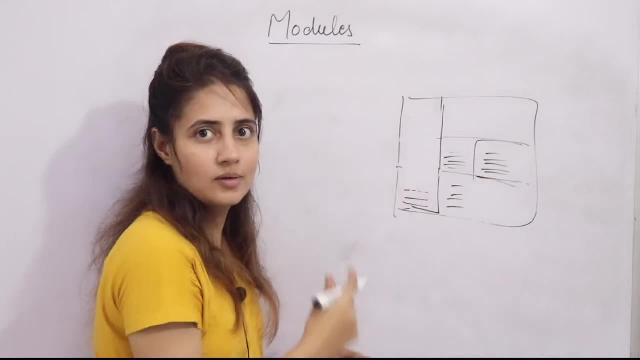 show you using import keyword. That is very simple in Python, right? Same like if I want to take my t shirt from here and I want to put here, put here. So I just take my t shirt here and I can put here. It's like just importing, right, Importing the module or importing something. 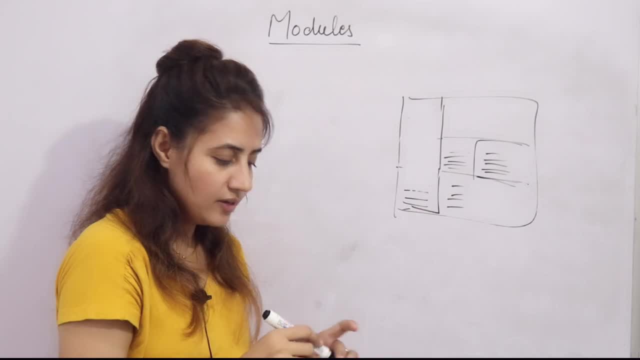 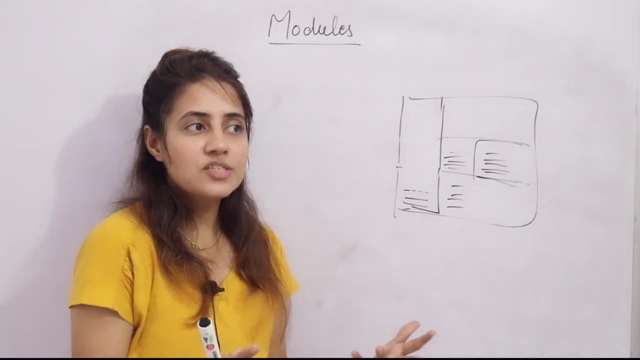 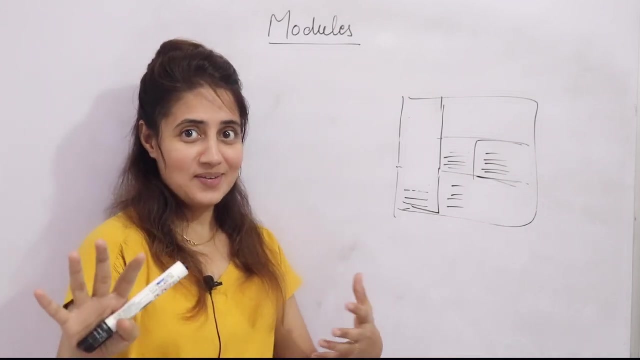 from any other file, Right? So first thing, this for easy maintenance of the program, right And okay. now next next reason is: why do you need modules? Let's take one more real life example. I hope you are, you are able to relate this example also. See, I personally love that roasted. 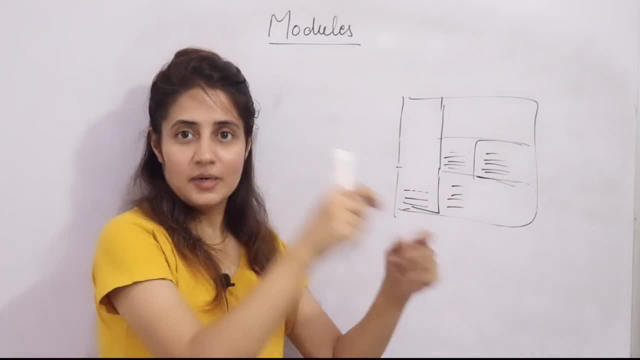 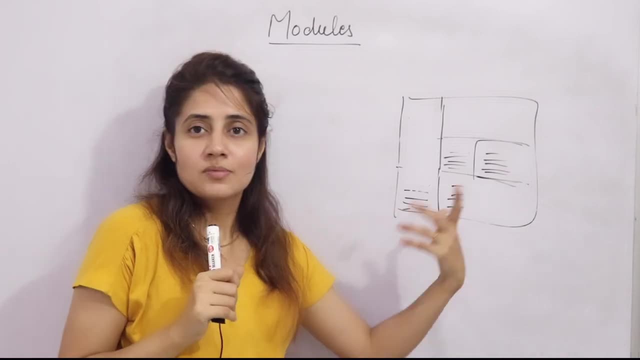 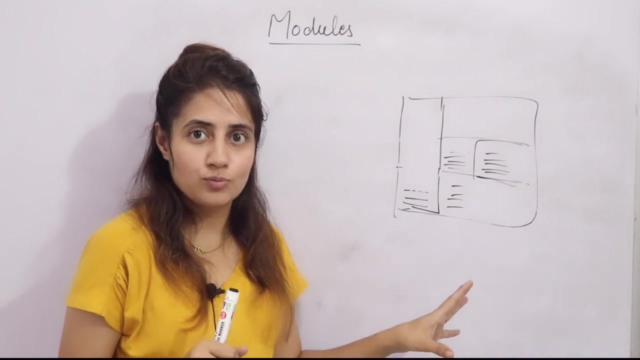 cumin powder. I put that powder in buttermilk or curd or in. if I have raita, then also, I just sprinkle that powder on that raita and some snacks also, like chaat or anything, then also mix that powder, you know, in that chaat also right. so what is one? 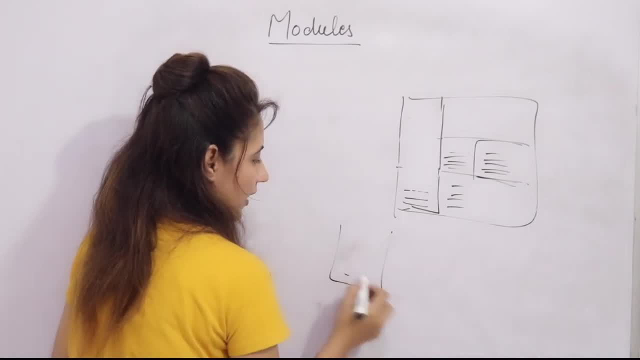 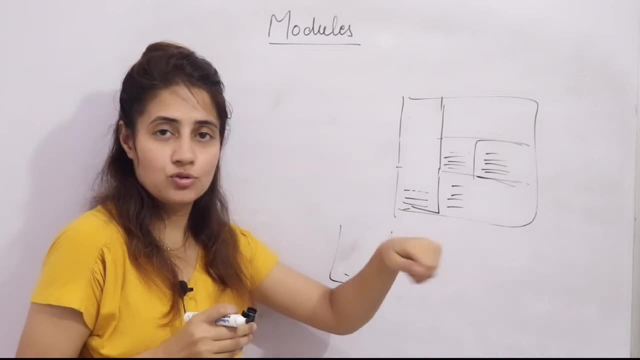 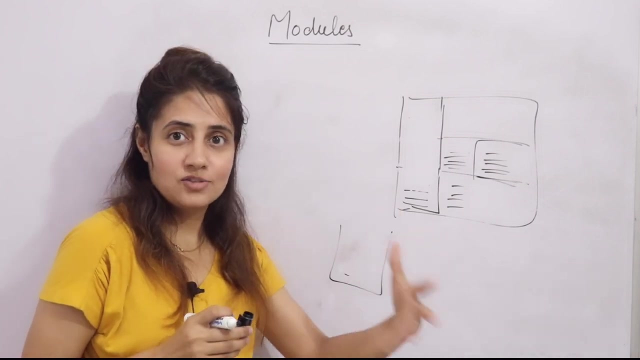 process. suppose I have a buttermilk. today I'm going to drink buttermilk chaat, right. so what I'll do to make that powder? I'll just take cumin seeds, I'll just roast those cumin seeds in a pan on medium flame, then I'll just, you know, make the powder. I'll just grind those seeds and that the 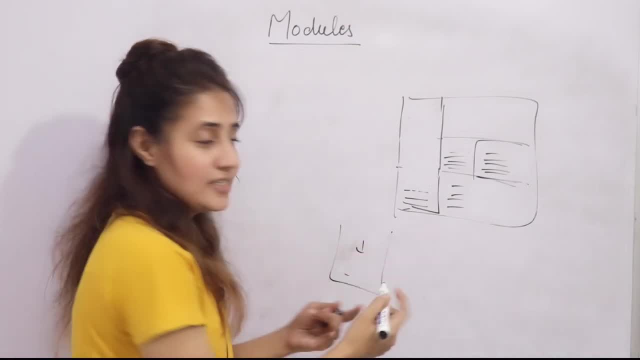 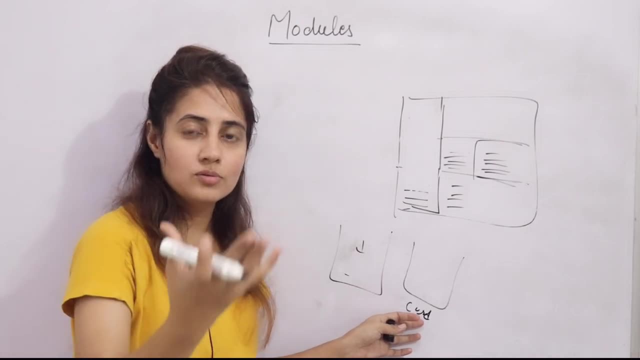 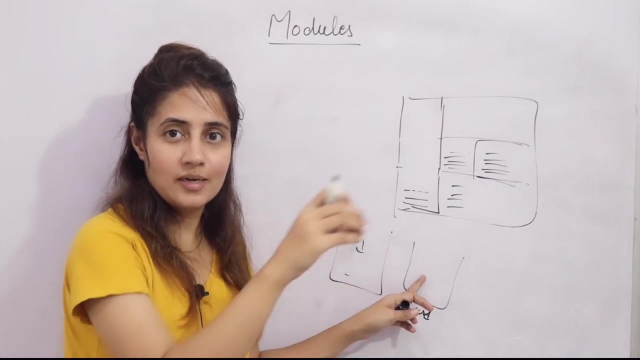 powder and then I'll sprinkle that powder in my buttermilk on the next day. I'm, I'm. this is good, I'm going to put. I just want to, you know, use those powder in this curd. also same process. I'm going to repeat: take a pan cumin, take cumin seeds, then I'll just roast those seeds and grind and then the 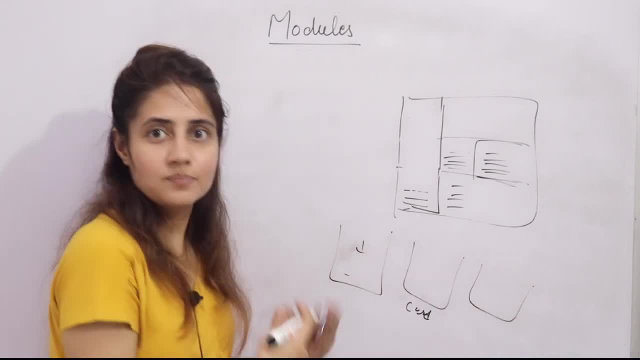 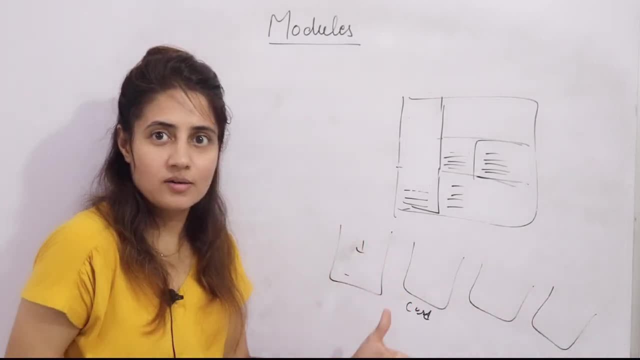 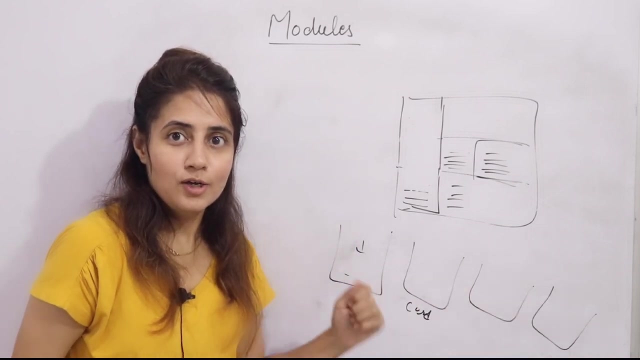 powder I'll use, I have next day on. I'm having raita, for that also I have to do same process next day suppose I'm having some snacks, some chaat, these kind of thing, and there also I want to put those powder- cumin, roasted cumin powder. so the same process I'll repeat. right, so this roasted cumin powder, I'm 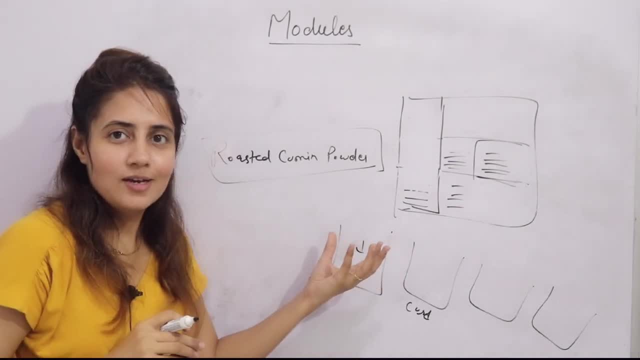 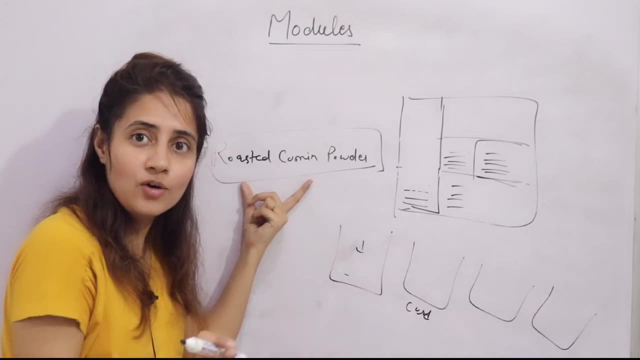 using frequently, right? so rather than repeating the process of making this powder again and again on each day, what I'll do is I'm going to make this powder again and again on each day. what I'll do on one day only. I'll take just one cup of cumin seeds and I'll make powder, and I'll just put that. 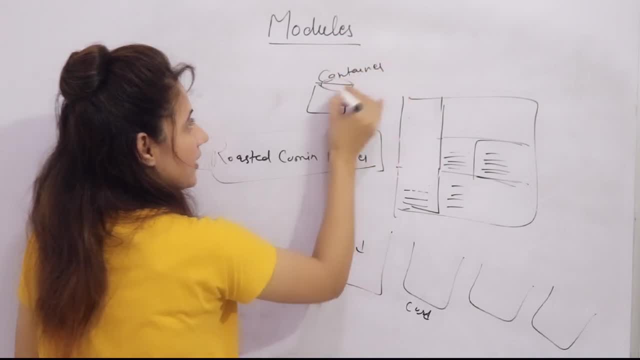 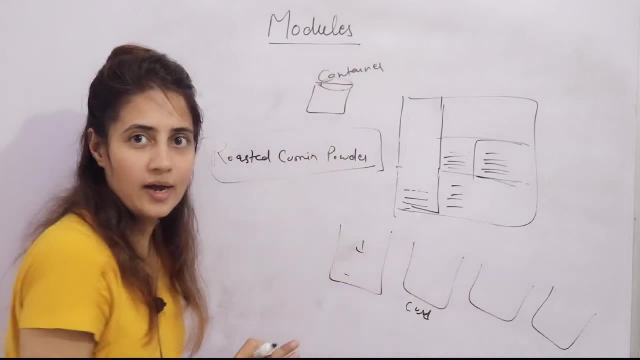 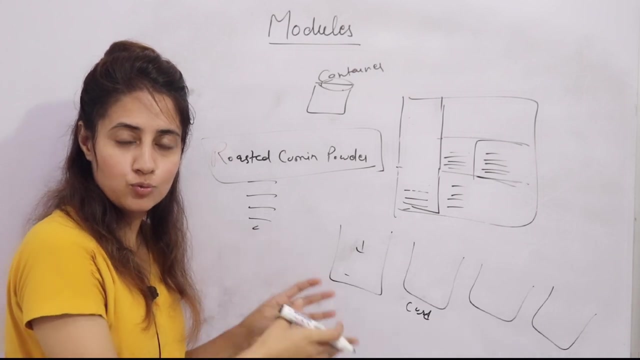 powder in container. now this is my container, so if I want to use in curd milk or anything, I just take this container, take some powder and use that, rather than repeating the same process of making this powder right. so I think that is very useful for me. if I do this process, you know if I, you can say a. 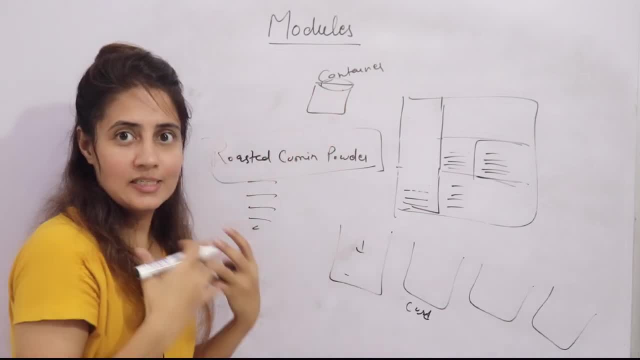 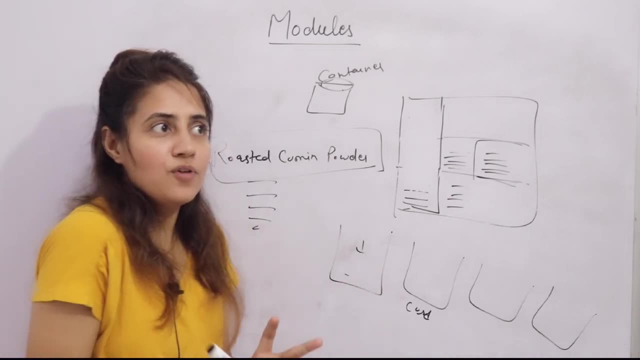 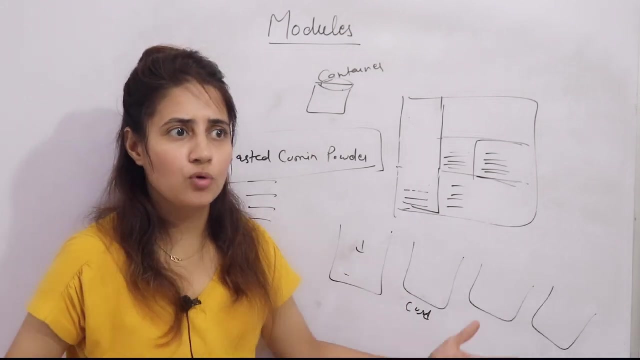 make the powder one day and just put that in a container. that is easy for me to use that again and again. right same thing, so same in programming. like if some functions are very handy or some functions are, you know, those are frequently used functions. we use those functions in many programs. 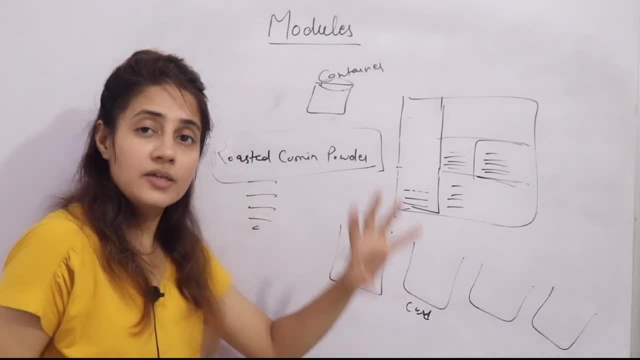 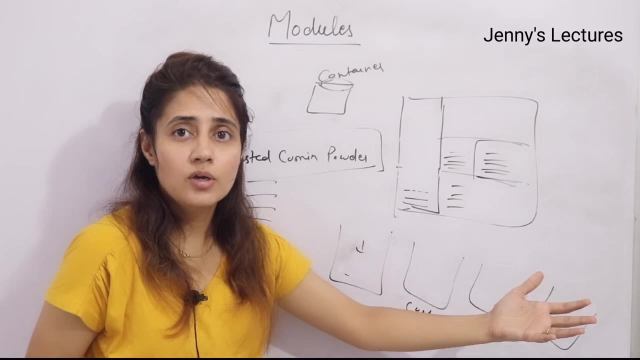 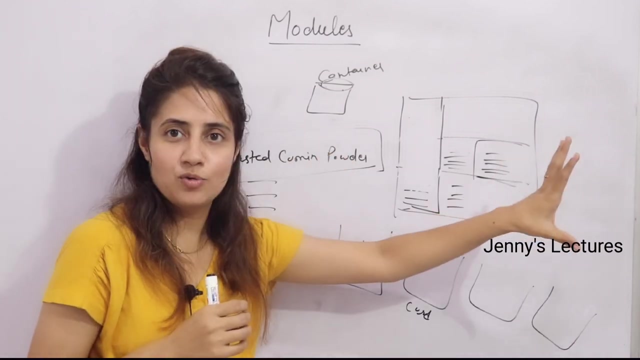 or in many projects, right? so rather than writing the definition of those functions again and again in each program, like for each project, what we can do, we just put those functions in a separate module, right? the definition of those functions in a separate module and in whenever you want to use. 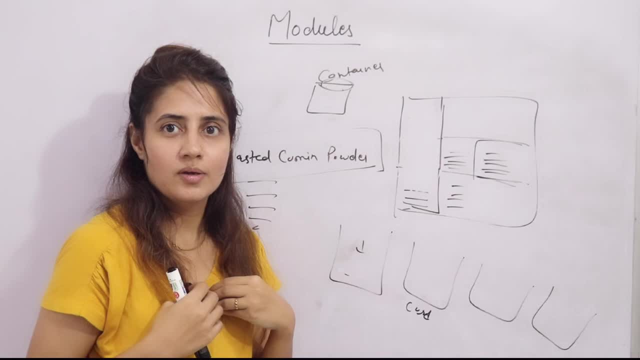 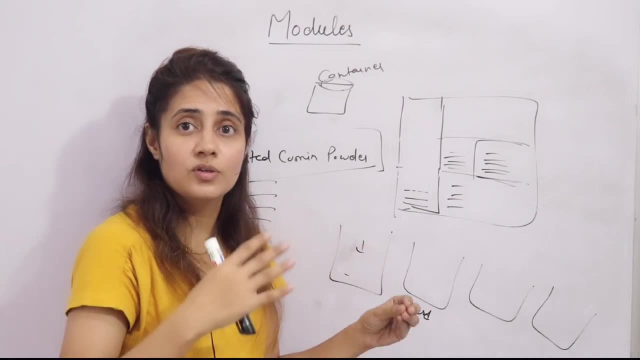 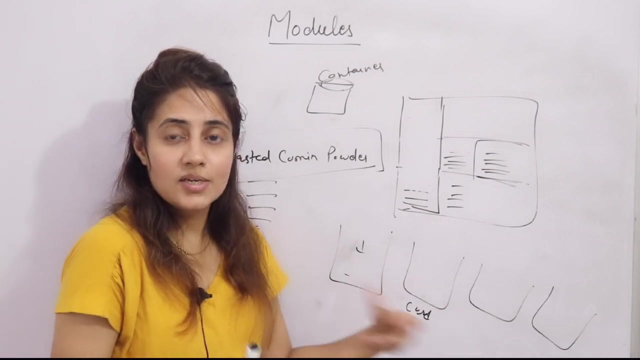 like in my project. i want to use those functions, so i just import that module. my friend also want to use those functions, so my friend will also import that module only, rather than writing the definition of the function again. it is time-consuming as well, right as well, as it is increasing the code reusability. okay, so i guess now you are. 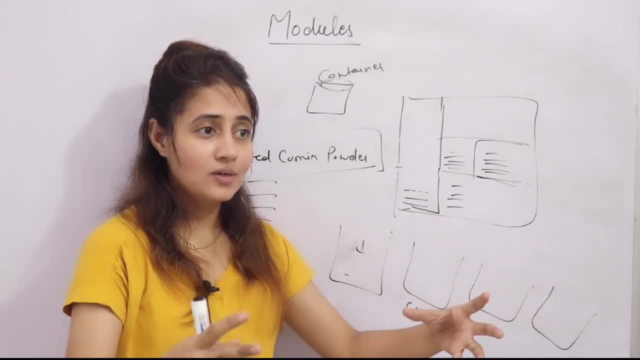 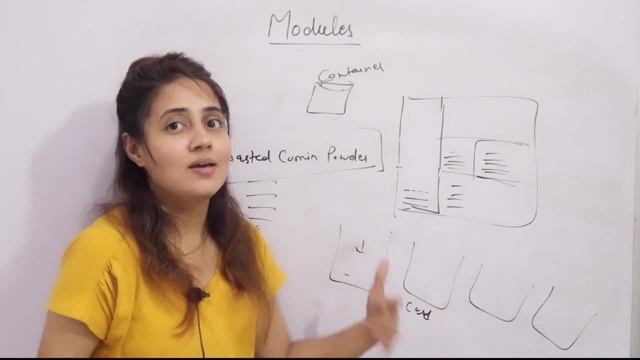 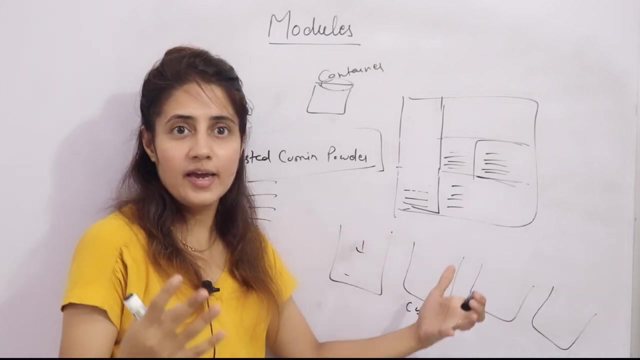 able to relate these real life example with the need of modules in programming. i guess so. if not, you can just let me know in comment section. i'll just try to improve my quality of examples- real life examples, right. okay, now i guess it is clear to you guys why we need modules, right. first, it 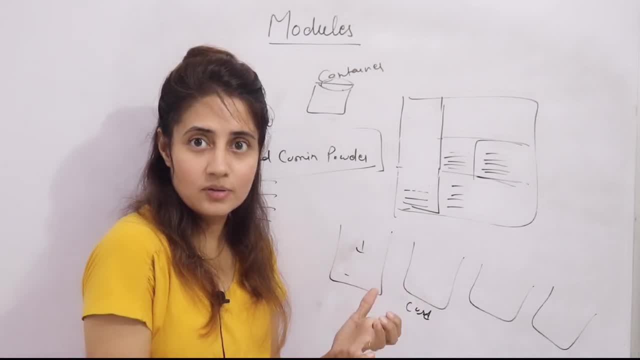 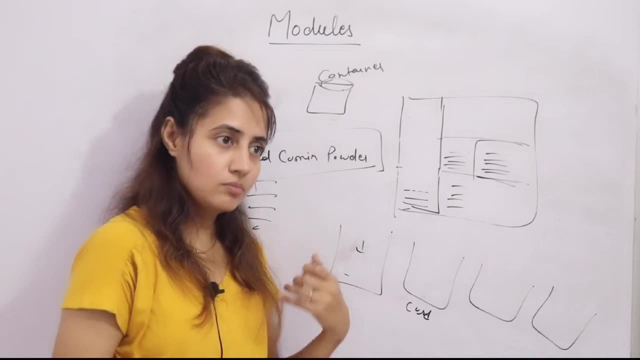 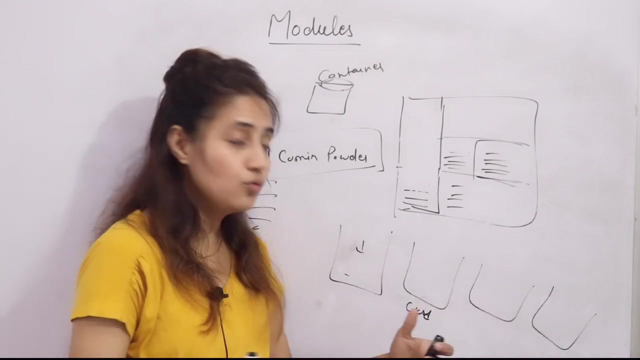 will increase the code reusability. obviously the time would be saved, time saving. next, the program or the project would be more manageable or easily manageable or maintained. you can, we can easily maintain that project if that is divided into separate files, right? or you can say it would. 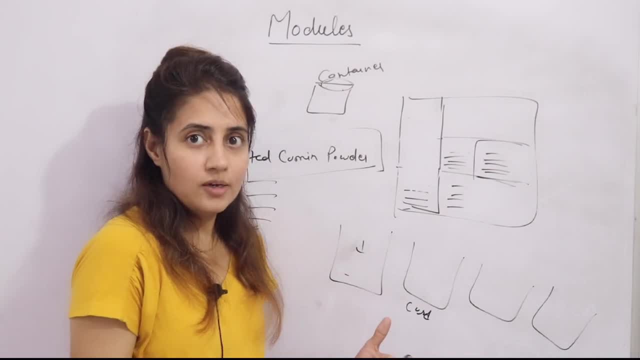 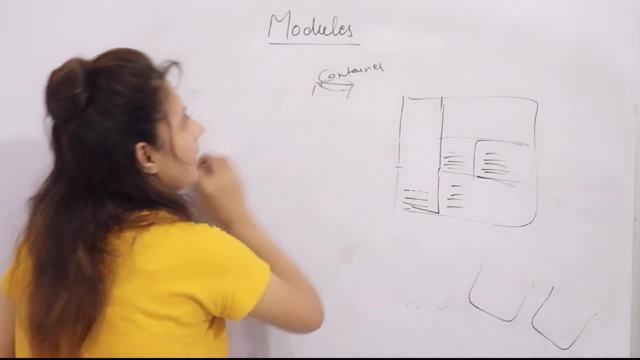 be definitely more readable, more understandable, right. so these are. you can say, some benefits of using modules. or you can say: this is what in need of modules. now we'll see types of modules. there are two types of modules, three types of modules, sort of you can enter or expand. you can say: 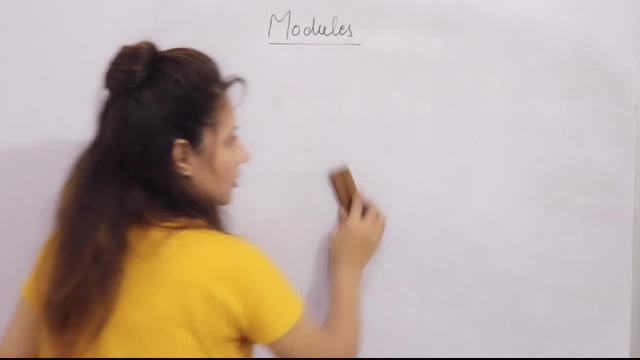 module you you can also up into module in your module. you can see which module or module is cooked place within different modules. so basically перекoli. i will also say i'll just hold for a second winner: built in as well as you can create your own module, so built-in modules like math, random and many. 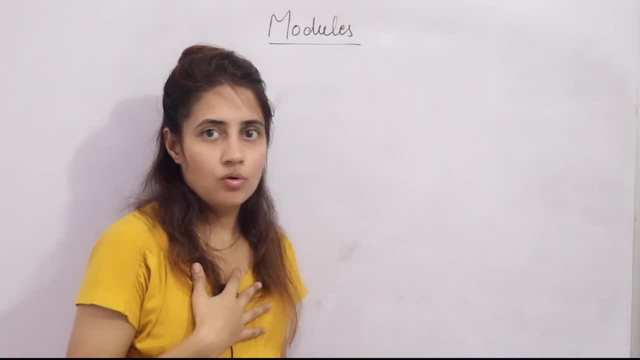 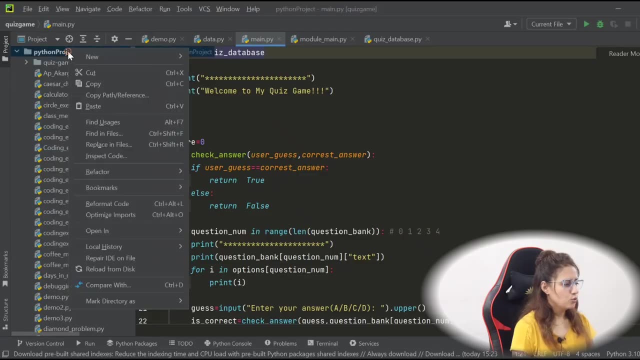 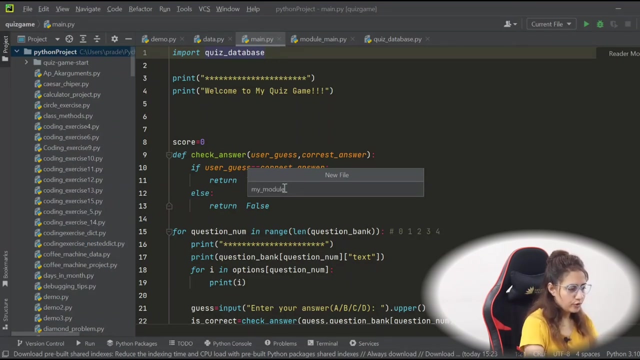 modules. i'll show you those built-in modules also, and we can create an our own module also. this thing we will see with the help of program, right? so let's do some practical, okay. so let's create a new file here, in this project only, and, for example, i'm just going to give it my module dot. 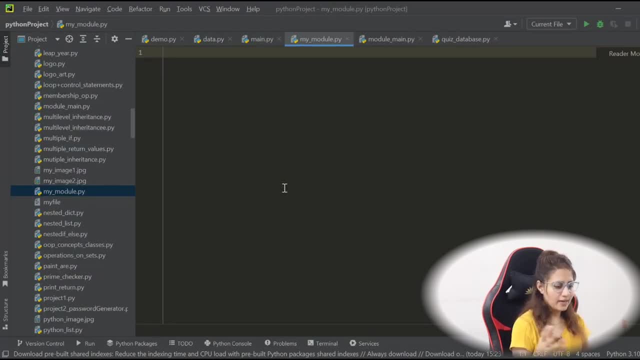 py, any name you can give. i've told you like every python file acts as a module, so module obviously having dot, extension, dot py. right now, in this we can have many thing, like maybe definition of some functions, classes, some simple statements, some simple variable, anything right. so in this module 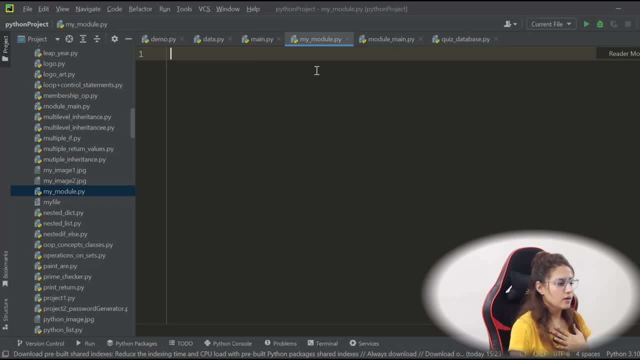 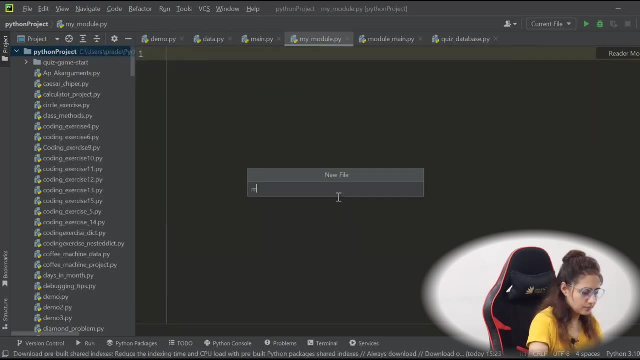 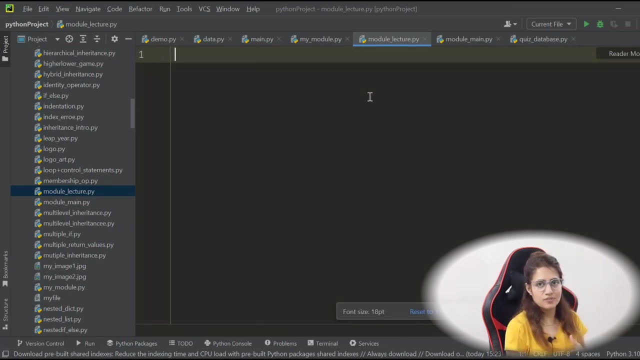 or right now, in this module. i'm not creating my own module, let's. let's have, like not my module, let's have a new file and i'm just naming it: module underscore, lecture, dot py. so first there are two types of module: built-in and obviously user defined modules. so first we'll see how to use built-in modules. 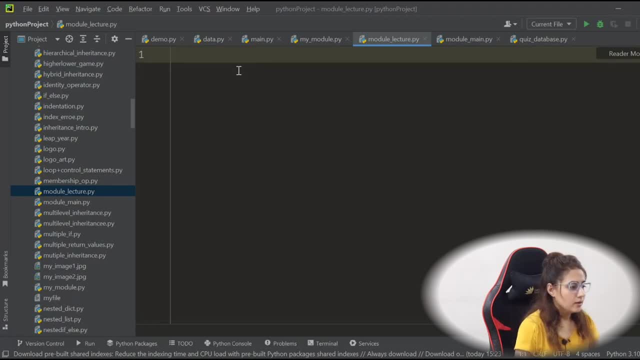 these are already defined right now. if you want to check out what are the built-in modules, then we have a function, we have help and then some argument you need to pass. so i'm just passing modules and and and i just want to print the what are the different modules i have? that's it, and this thing you need. 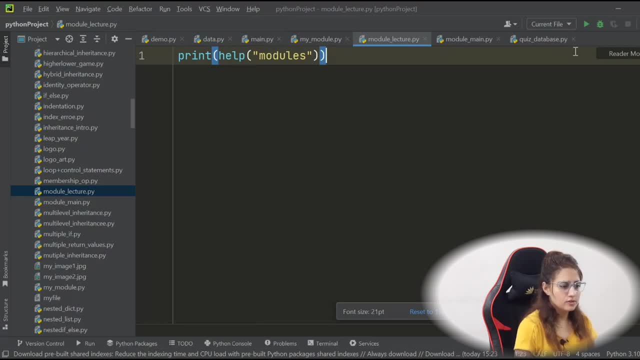 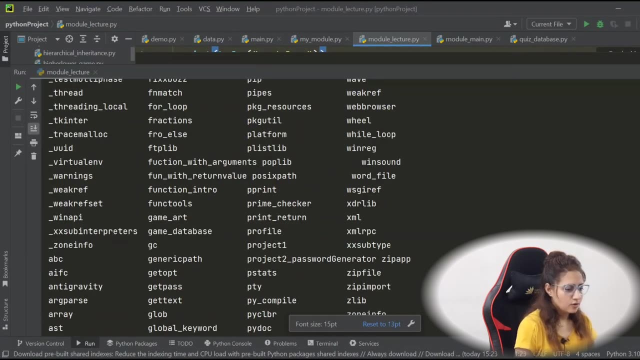 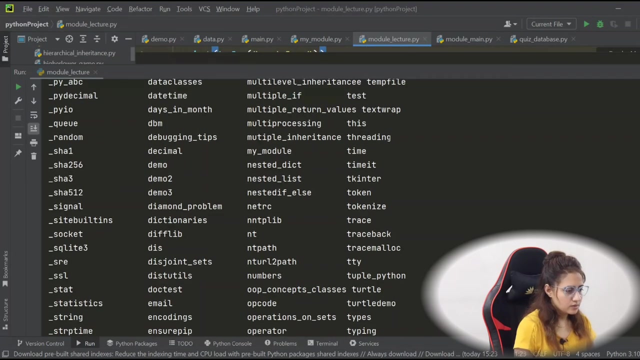 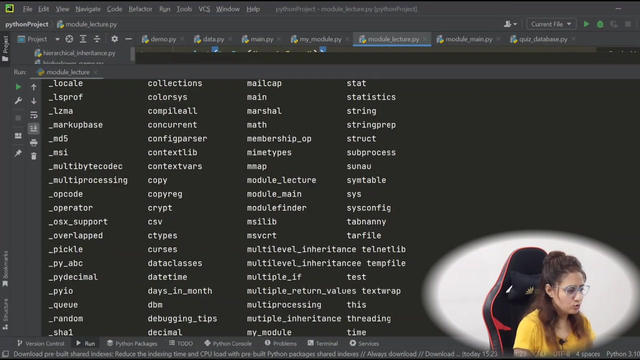 to write down the help function and bracket in as an argument, modules. let's just run this and see we are having these number of built-in modules. so i guess some modules are. see, we have, i guess, a random module, total module, and we have used math module, random module. these modules we have used right. so if you 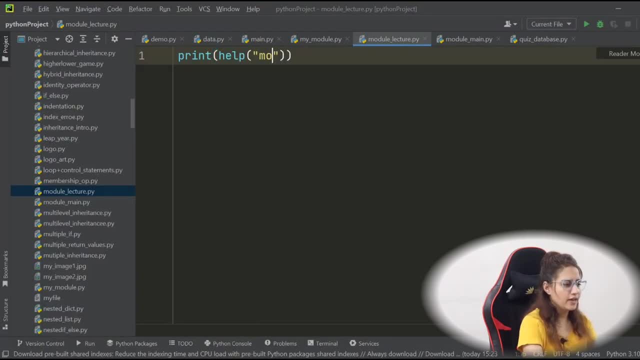 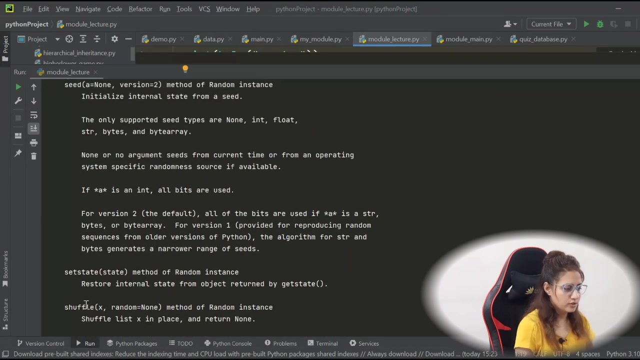 want to check out if in math module what we have or any module what we have, then we can check out, like i'm just going to check out in random module what we are having. so let's run this. see these functions we are we have in this random module: see shuffle seed. 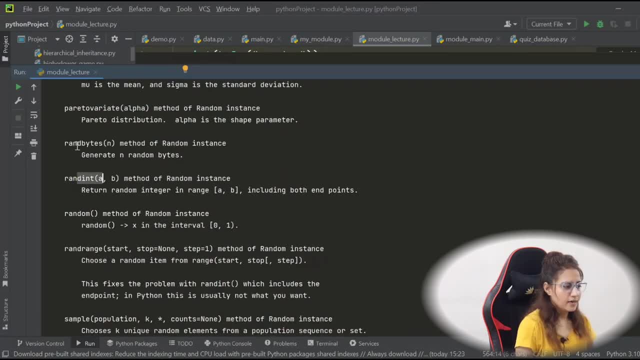 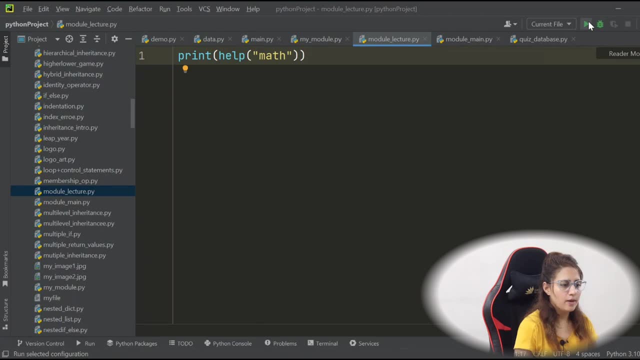 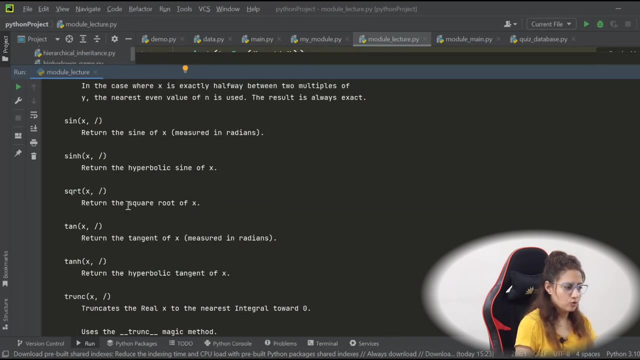 these functions, some function we have discussed, right, random brand, and these functions we are having, functions we have. okay, now suppose, if you want to check, like in math, what I'm having in math module, I am having the data we have- value of e, value of pi- having in math module, right? so how to import this module in your file? you just 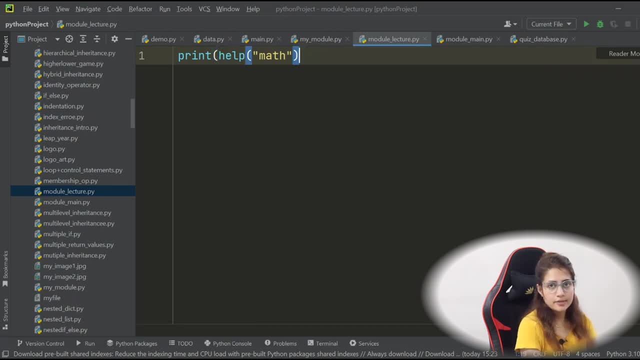 have to use import keyword and the name of the module: math. that's it now. this has given you the access to use whatever the data or the functions in math module you can use, right. but it's not like that it has incorporated or imported all the functions and data. no, it had just incorporated or inserted the. 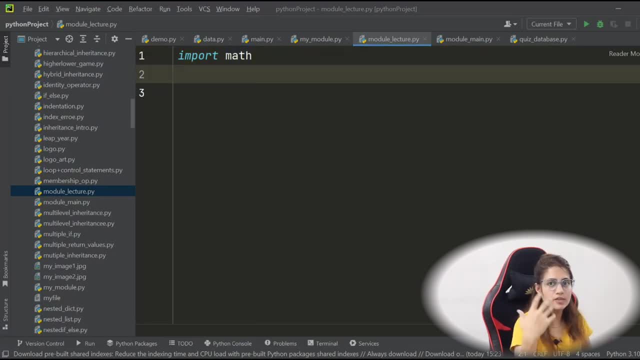 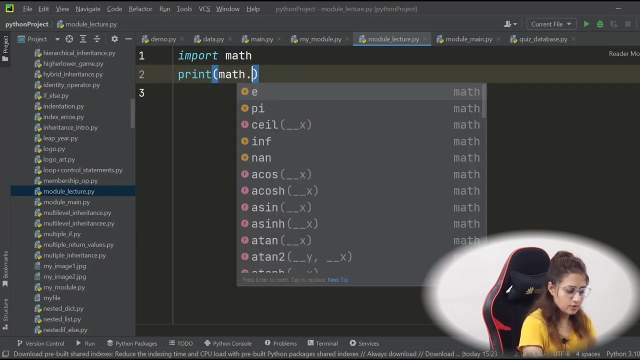 name of the module math. to use those functions and those data you have to use the name of the module first, like if you want to print the well well value of that variable, what we have seen, e, one variable, e that well variable. so you have to use first the module name, math dot c. we have e, pi, inf, nan and this. 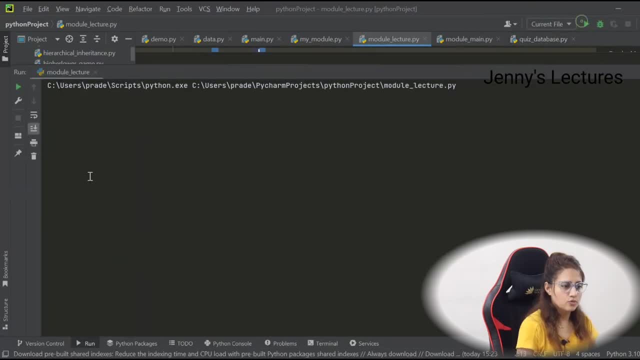 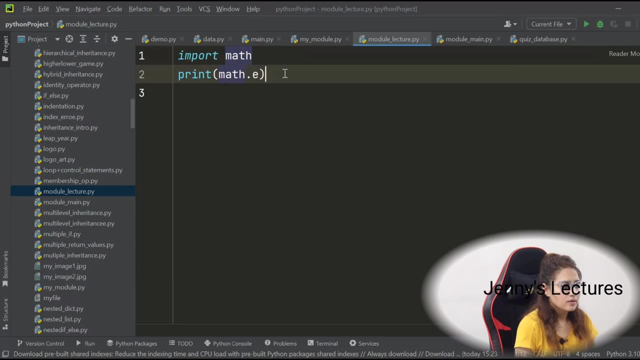 we can use. so I just want to print value of e math dot e. let's run this and see. this is the value. now you can access everything, right? so this is how you can import built-in module. now we are going to create our own module, right? so I? 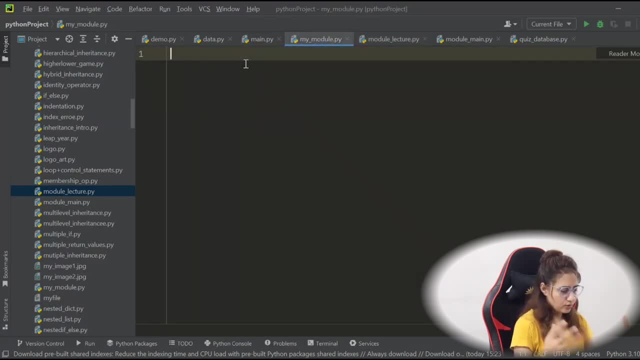 have my module dot py. so here I'm going to. you know, I'm going to take first a variable, suppose a is equal to 10, and then I am having a definition of some function. may be like like area of square, and just need to pass one side, so one. 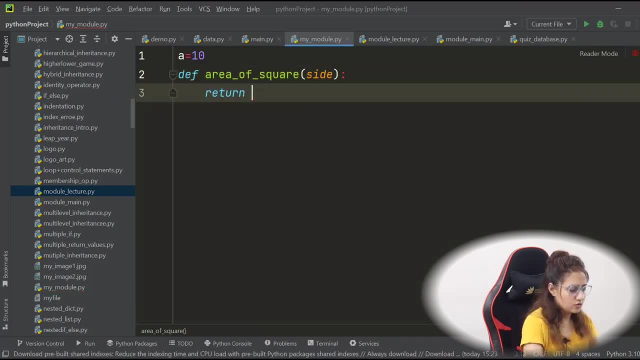 argument, like I'm taking the variable name side and it is just a returning and the area of square is what I think: the side square, so power of square, so 2.. Then I am having one more function maybe, suppose calculator, and I'll just pass here. 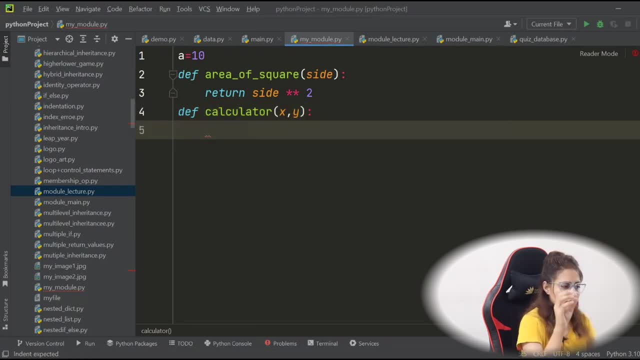 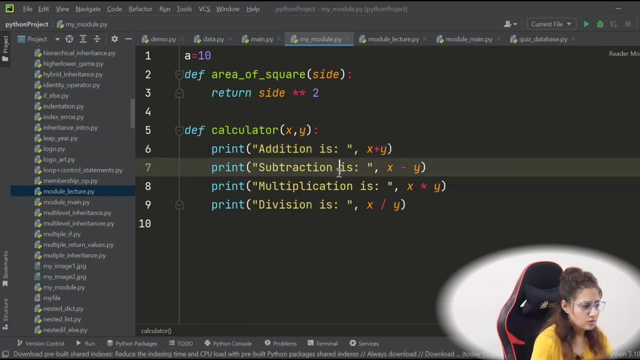 two argument, x and y, and to just print addition, subtraction, multiplication and division In this definition of this function. I am having this addition, subtraction, multiplication and division right and only one function. this I'm having. so that's it. I'm having only two functions and one. 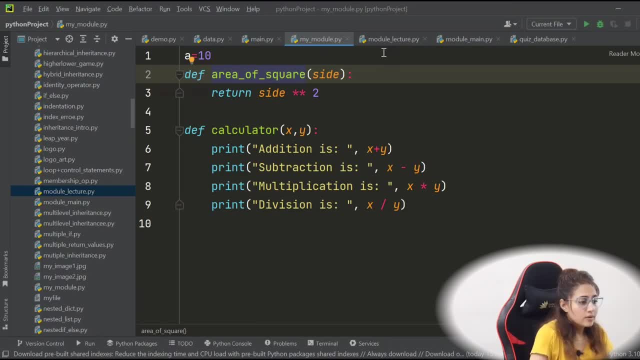 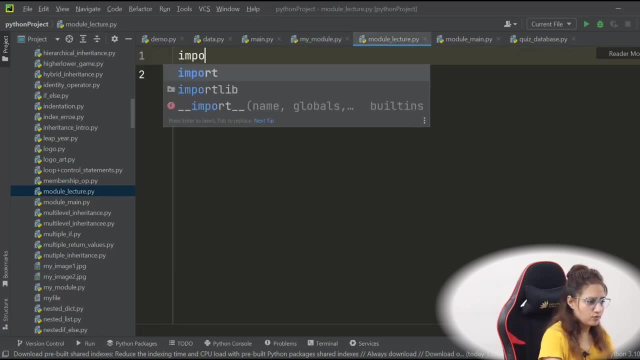 variable. okay, So now in my module, in another file, I can import this module. so how to import? you just have to use this import keyword and my name of my module is my module, my underscore module. right now I can use anything: this function, this function and this variable, everything from. 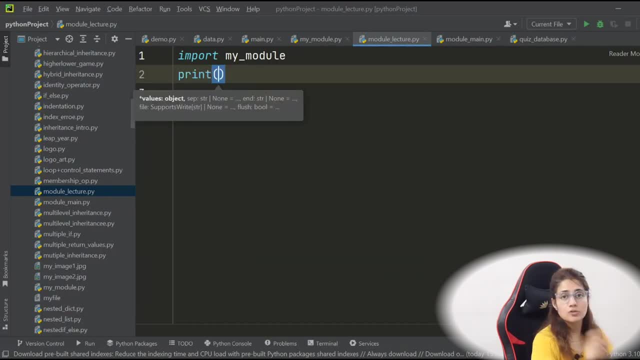 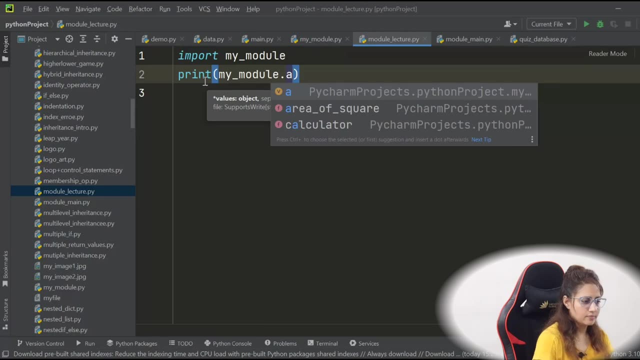 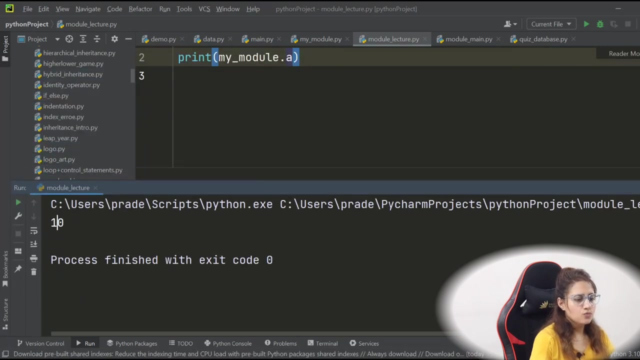 this module. So suppose I want to print this what we can say value of a, that variable. so first you have to use the module name, dot a right, and let's run this and see it will print 10 right. this is one way to import module. another way is import module alias name. suppose your module. 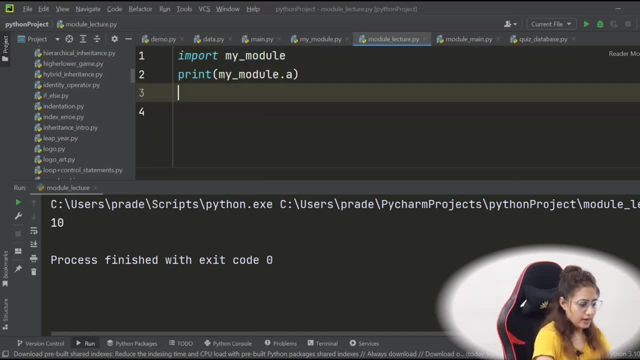 name is a big name, so everywhere, and here suppose you want to call that function square, so my module dot square, area of square, and just pass one side and it is returning something. so you have to write here: print. okay, then again, I am going to, let's run. 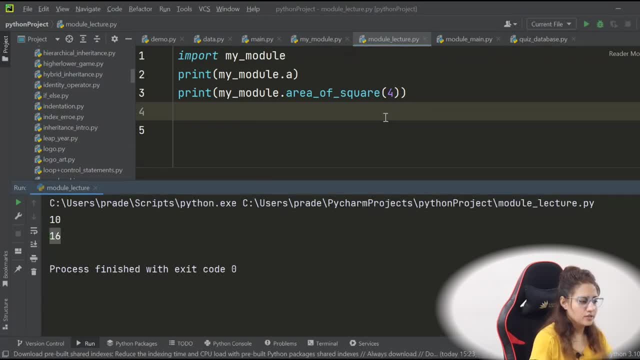 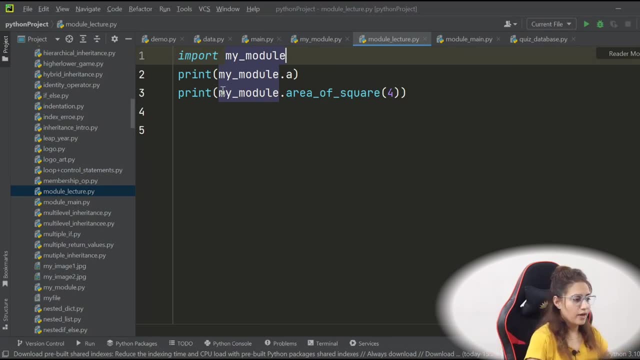 this: first see 10, value of a, and then 16 is area of square, right now if my module name is very long. so every time you have to use module name, then dot, then whatever function or variable you need to use. so a small name I want to give here so as an alias you can import that thing. so 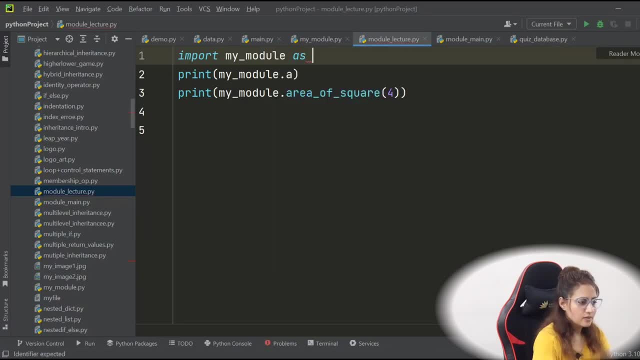 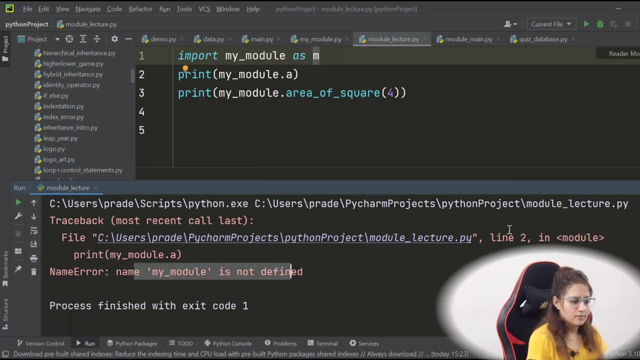 the second way is import that module name as small name I can give like m only now, rather than my module. now my module name in my file is m, so now it will give error if you run this. see name. my module is not defined in line number two here. my module dot a, now it is m only. 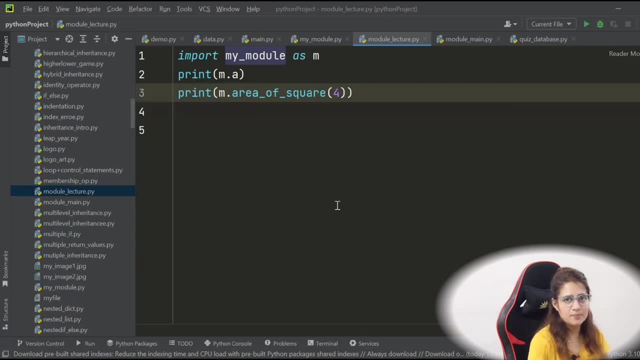 it's not my module, because I have renamed this. it's m now. okay, it's run this. see now 10, 16.. so this is second way. third way is, specifically: I don't want to import everything from my module. suppose I have 10 or 15 functions, but I just import one function here. I 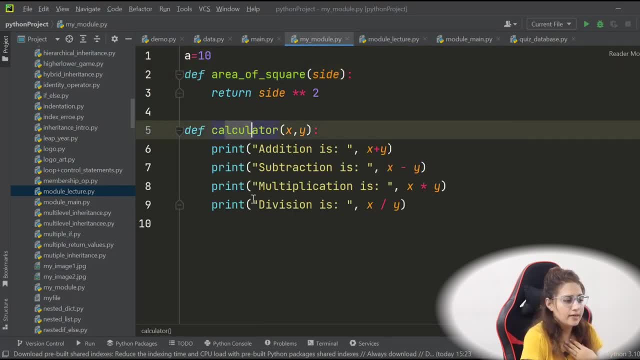 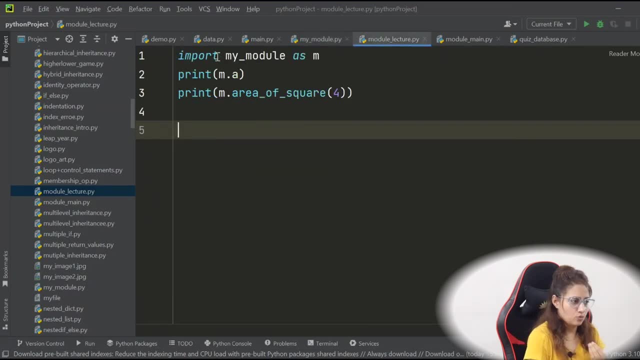 have only two function, but I just want to import or use only calculator function. so rather than importing everything, only one specific function I want to import. so therefore, for that you have to use from keyword, so from the name of the module, and then I want to use from the name of the module. 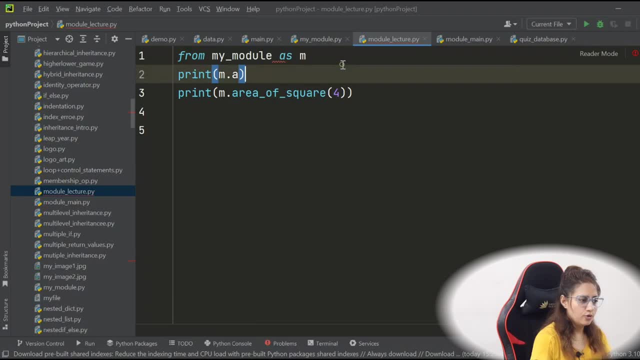 this is my underscore module and what you need to import import only calculator calculator. so now you cannot use here a or area of square, because we, you have just imported calculator. so let's just comment out these thing and call the function calculator calculator and just pass: three comma uh, three comma two. 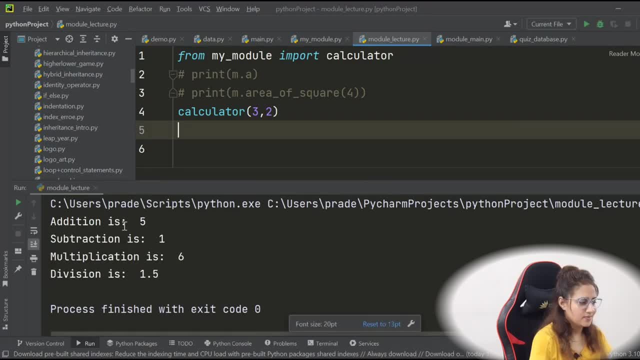 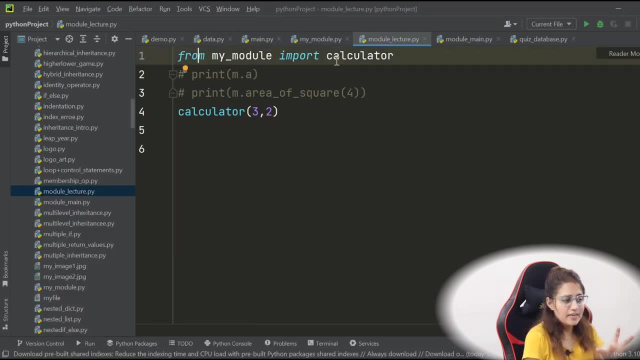 these two values. let's run this addition, subtraction, multiplication and division right. so if you specifically import calculator, no need to write down here the module name dot. simply you can use the function name calculator, that's it, or this calculator, this also you can give a separate name or you can say alias name, like calculator, as. 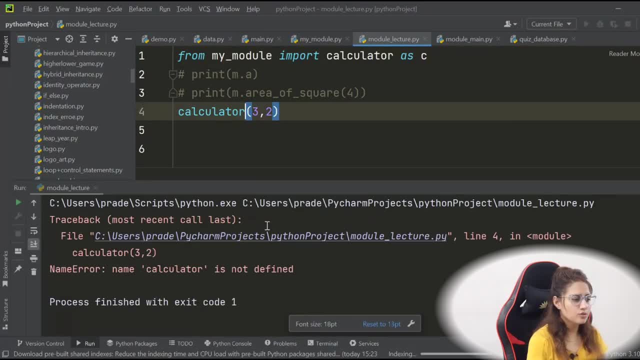 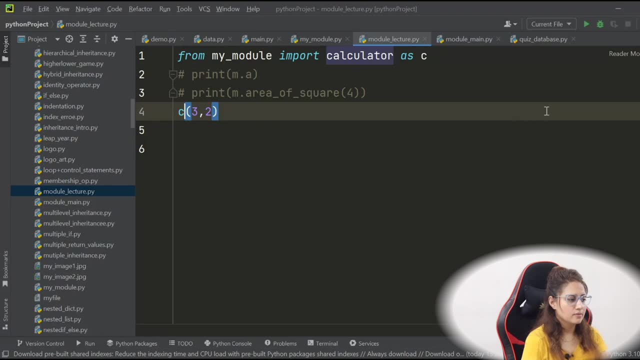 c. so now, rather than calculator, you need to use c, because now calculator is not defined, because I have renamed this as c, so you just need to pass here the name. function name is c like this. so when you use this aliasing concept, if the module name or the function name is very long, 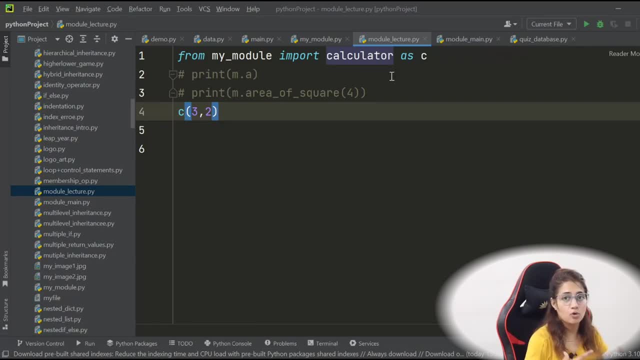 so you can use aliasing concept rather than writing the same name again and again, the long name, right. but one problem with this thing is what? if you want to import a specific thing, then the problem is suppose i want to, and next thing? next thing is what i want to import, as well as the variable. 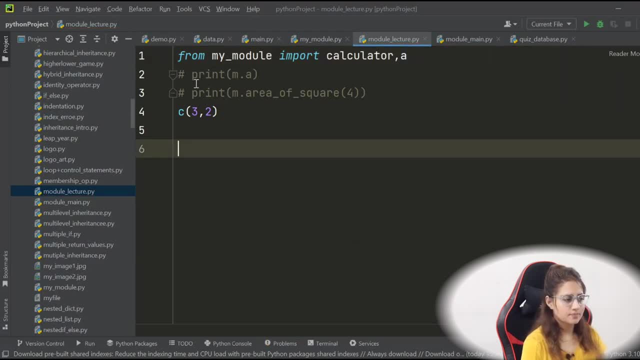 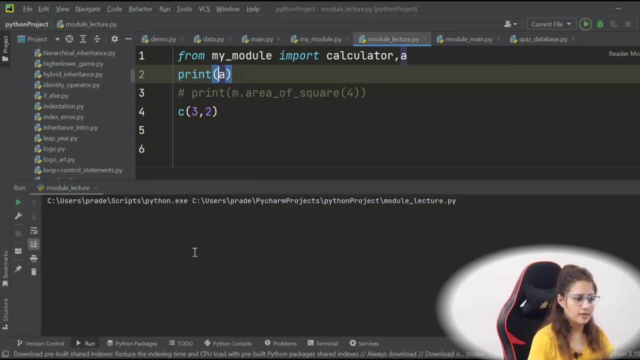 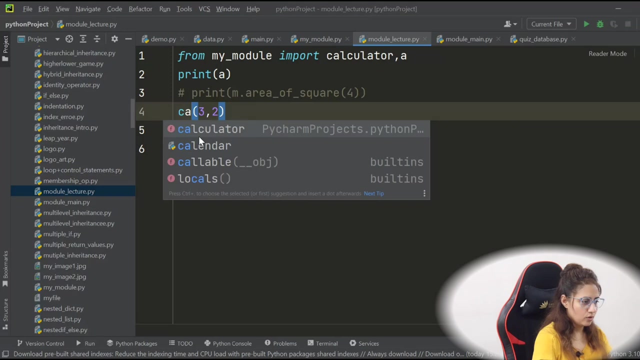 name a, so just write down comma a. so now it will work. fine. you have to simply print a and c, a. let's run this. okay, name c is not defined because we are using, not aliasing. now we are using here what the complete name, calculator, right, c, 10, and then definitely this calculator function, right. 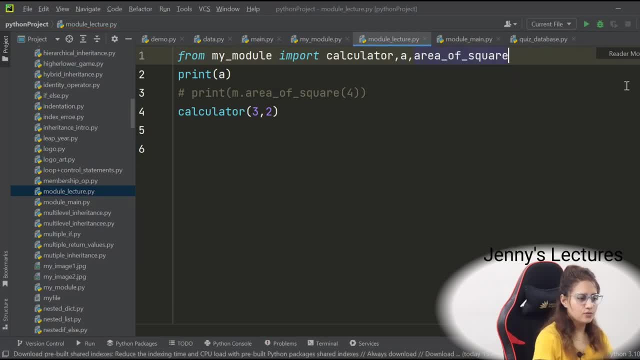 if i want to import area of square as well, so for my area of square, or rather than writing here separate, separate name of the function and variable name, what we can do simply, we can put here as a strict: so now, specifically, it will import everything, a whatever is there a this function, this function, all the. 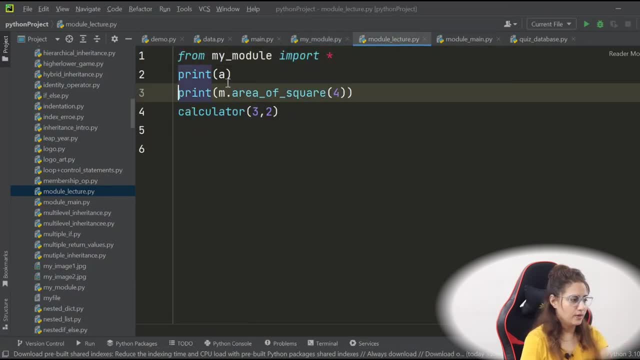 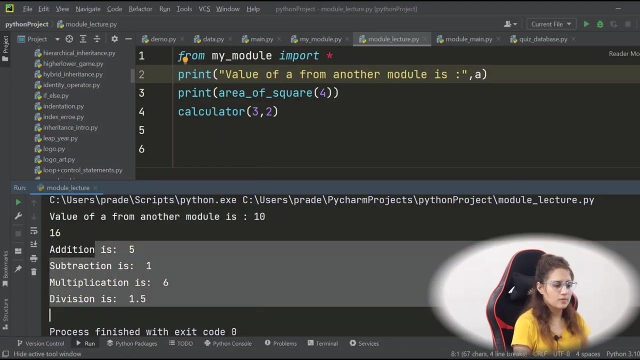 three things now. it will not give any error if you print this thing also area of square, or here i just want to print something like this like value of a from another module. is this? so let's run this value of a: 16 is area of square and this is that right. so this is another way of importing. 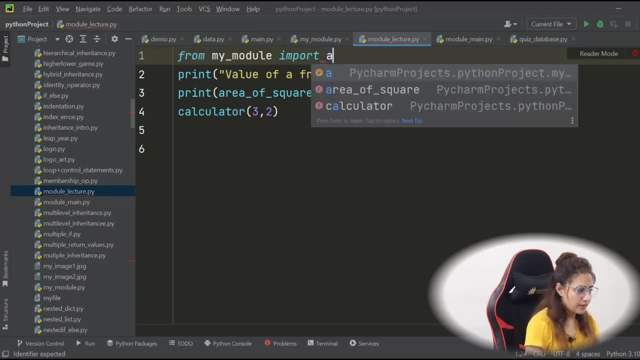 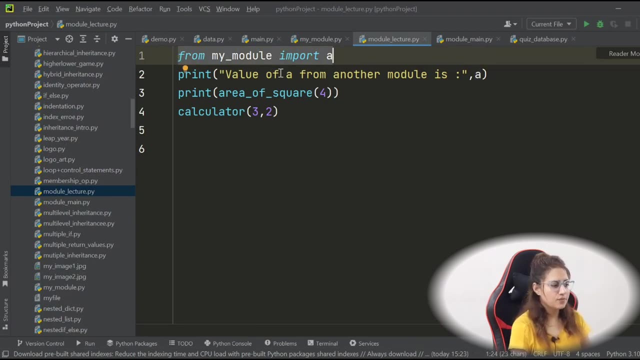 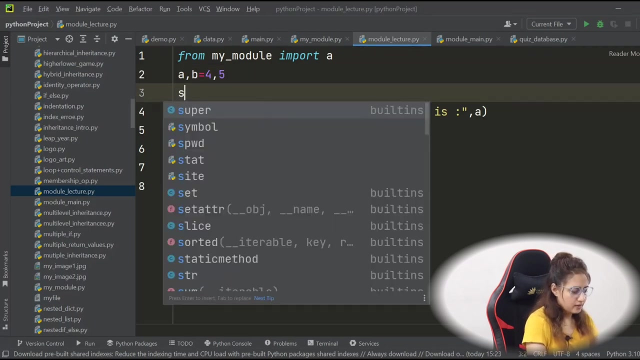 see separately if i want to import separate, like a from my module a. but the problem in this case or in this way of importing specific thing is what if in this file also i am having one more variable a, or suppose a comma b and equal to i am having 4 comma 5, right, and then i am having some sum equal. 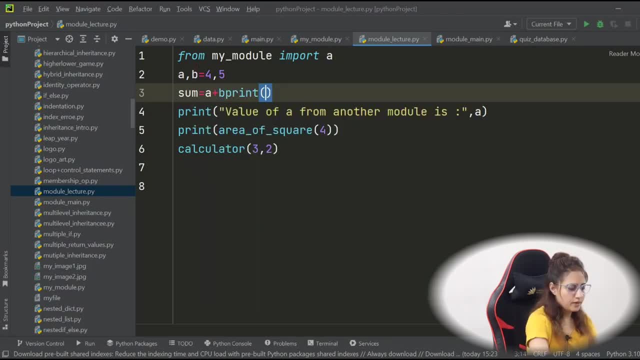 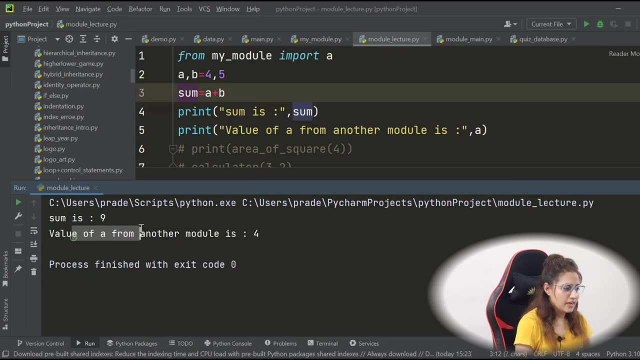 to a plus b. so again roaring, and just i want to print sum. see, sum is nine. fine, four plus five is nine. value of a from another module is four, but from another module value of phase ten. it is importing, it is just printing this a from this module, only a. but i want to print. 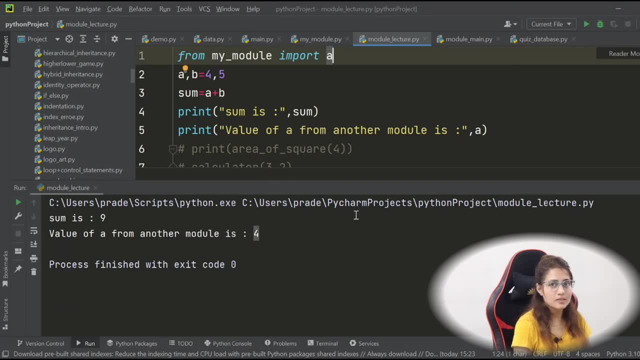 i want to access this value. so in this case it's compulsory to write down here specifically exclusively vehicle value only, because what is thatandoi would have given towards physical 수 used number. there are intentionally written to equal values such as position of minutes. not said this: a is from another module, from my module, so the name of that module, my module, dot a. 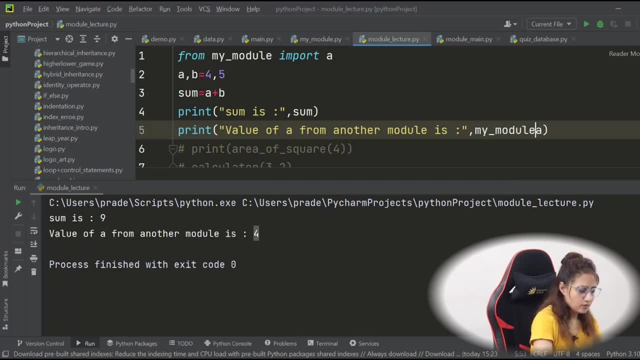 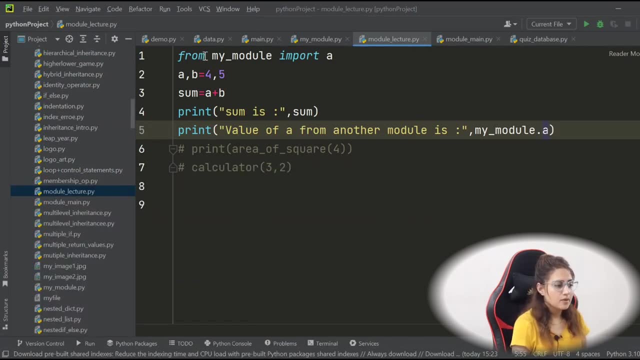 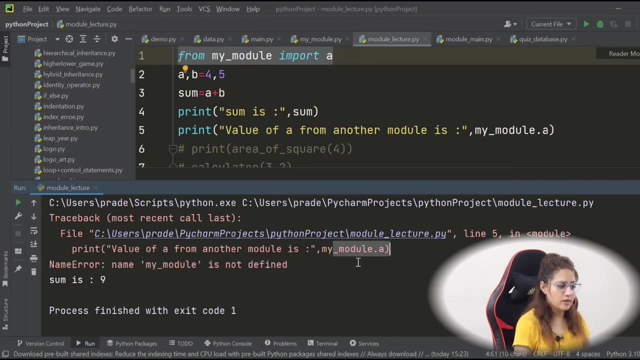 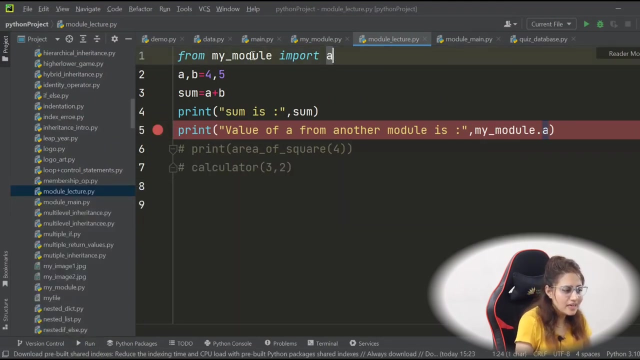 like this: my underscore: module dot a. but still it will give error because because we have used this way of importing this a. see, let's run this and i'll show you the error name. my module is not defined here. my module dot a in line number five: here my module is not defined because we have just imported this a, not the. 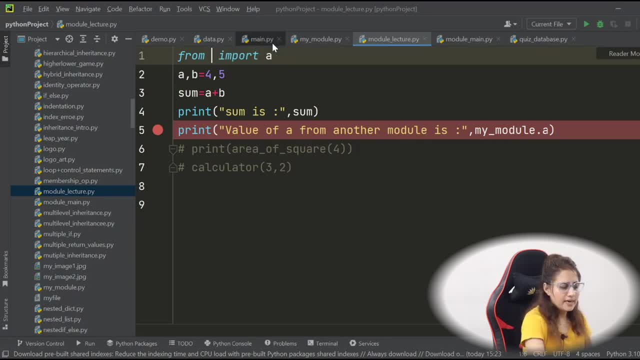 complete my module. so the better idea is what i suggest to use is import and the name of your module, my module and whatever you want to use now, any function or variable or anything exclusively. you can just tell i'm using this thing from my module. so my module dot a now run this.